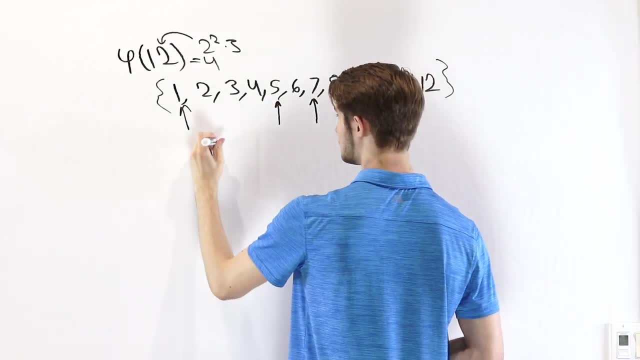 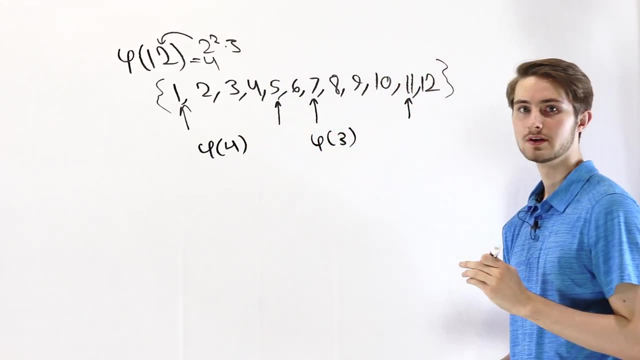 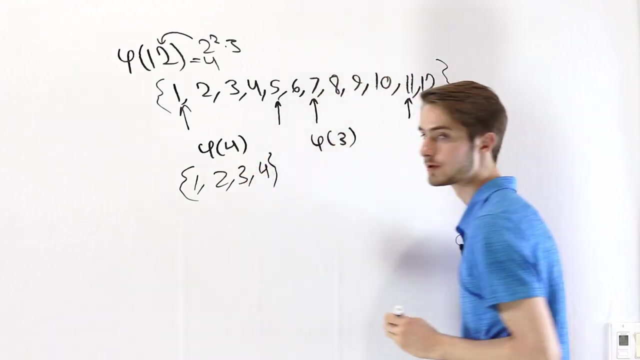 So I have another question, which is: what is phi of 4,, which is 2 squared, and what is phi of 3?? Well, we know that phi of 4, is going to be all the integers in 1,, 2,, 3,, 4, co-prime to 4.. Since 4 is 2 squared, 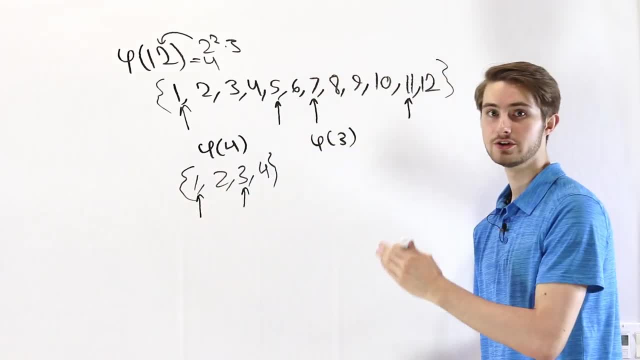 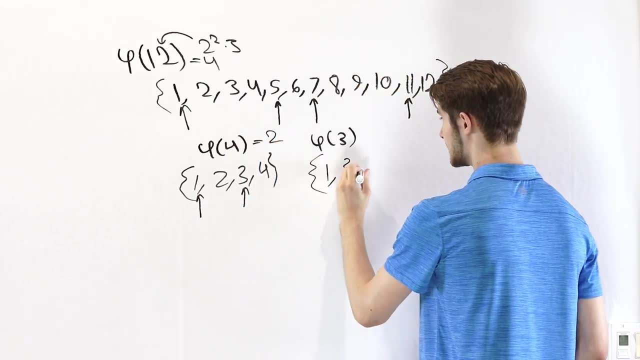 that's all the odd numbers. So 1 and 3 share no factors with 4, and that means phi of 4 is 2.. Similarly, for phi of 3, we're looking at the set 1,, 2,, 3.. So we want all the numbers in here that. 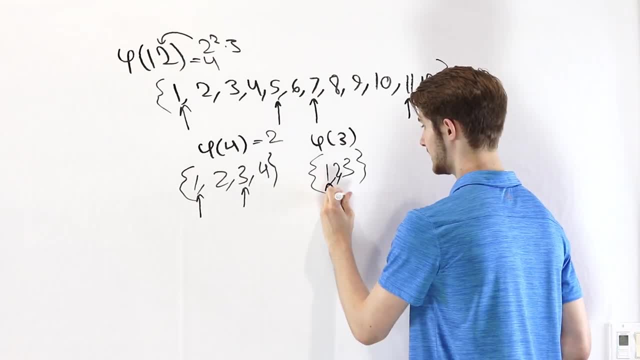 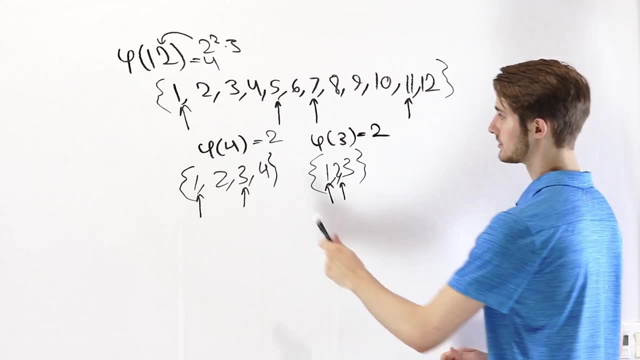 don't have a factor of 3.. That's going to be 1 and 2,, which means phi of 3, is equal to 2.. Now there's something interesting happening. Notice: phi of 4 is 2, and phi of 3 is 2.. 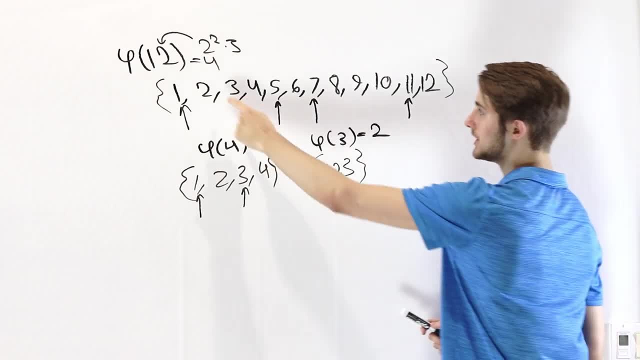 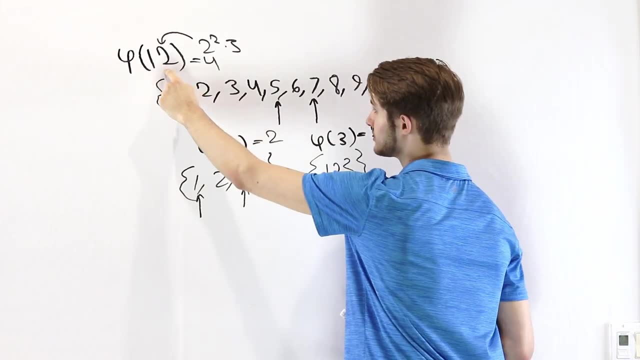 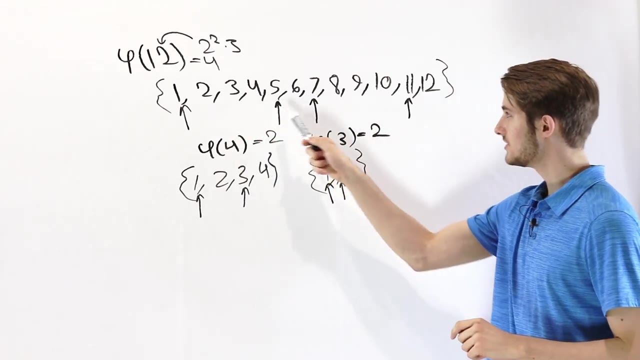 If we multiply these 2 times 2,, we get 4,, which is 5, 12.. So phi of 4 times phi of 3 gives us 5, 12.. That's a little bit odd, because these numbers that we see up here- 1,, 5,, 7, and 11,. 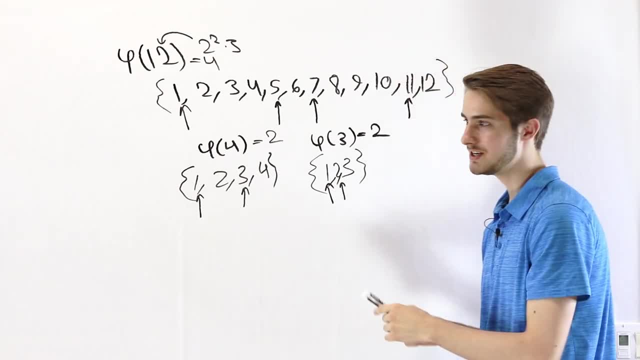 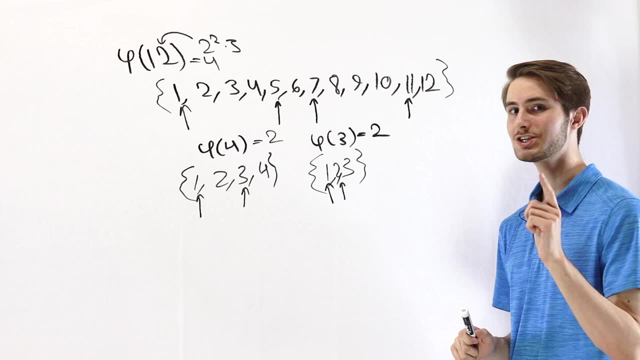 don't seem like they're really related to these numbers down here. These numbers are just 1,, 2, and 3.. Are they really related to 7, and 11, and 5? They actually are, and that's the interesting property that leads us to the proof of the. 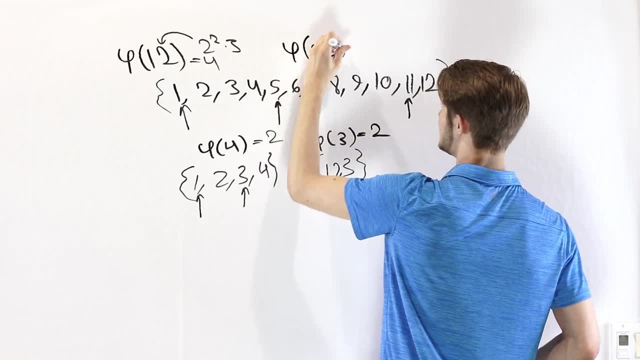 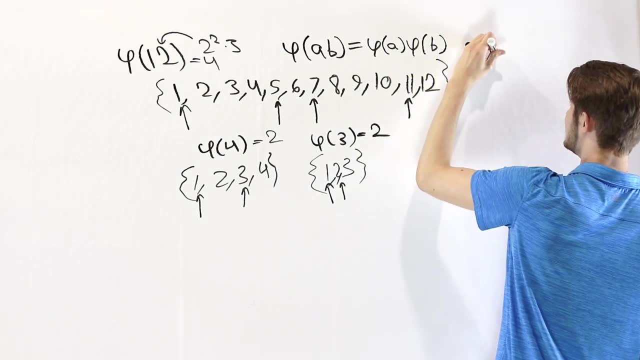 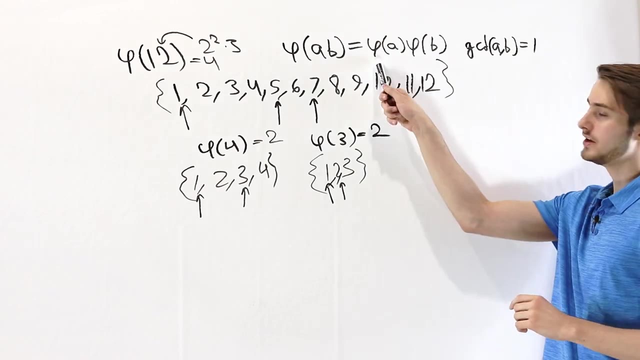 identity that phi of a times b equals phi of a times phi of b if the GCD of a and b is 1. In other words, if a and b are co-prime. This is what it means for the totient function to be multiplicative. 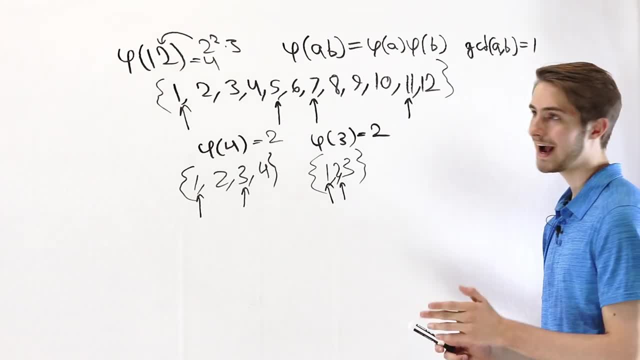 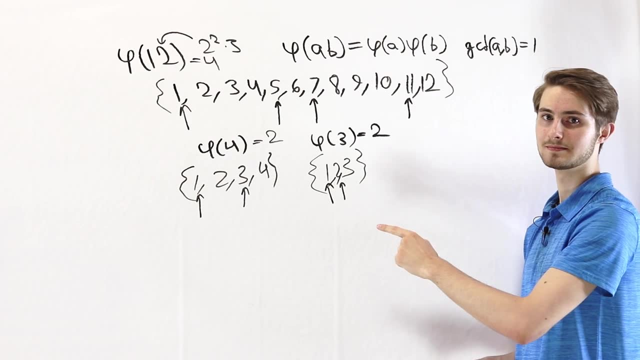 So what we want to do now is understand how these numbers- 5,, 7, and 11,- are related to these numbers down here, In order to prove that phi of a times b equals phi of a times phi of b. we're going to: 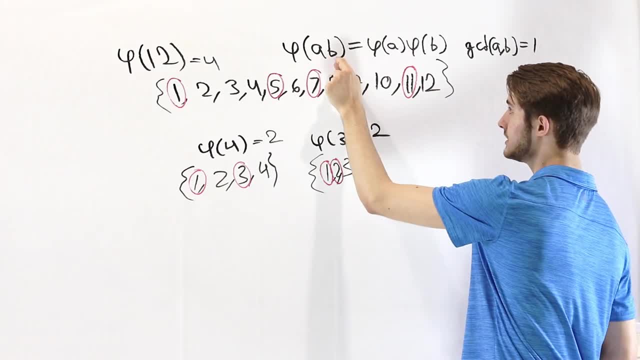 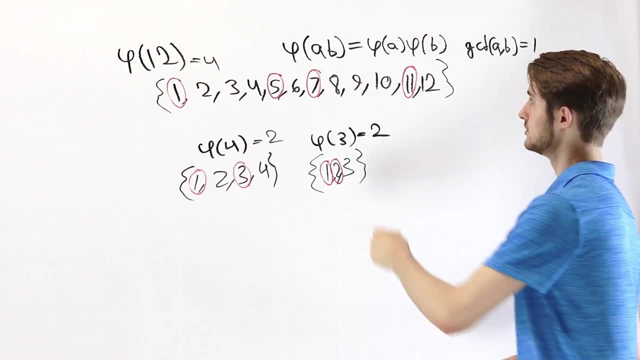 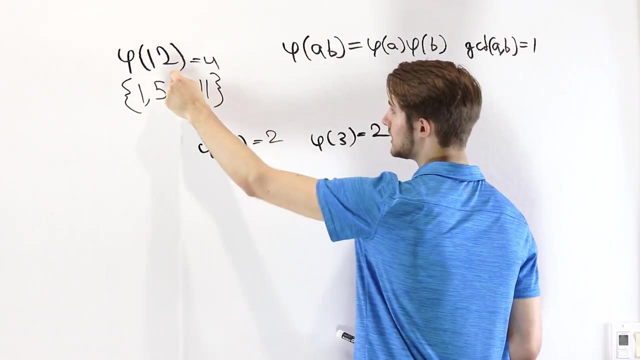 start by constructing this set of numbers that are relatively prime to a b. between 1 and a- b, The size of that set is equal to 5ab. It's the number of integers co-prime to a b. So in the case of a- b being 12, we have the set 1,, 5,, 7, and 11.. Those are all the numbers less. 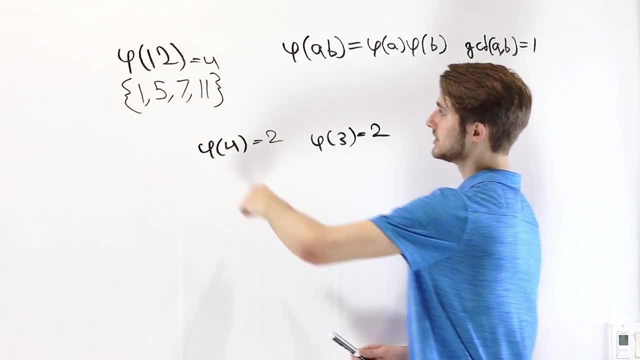 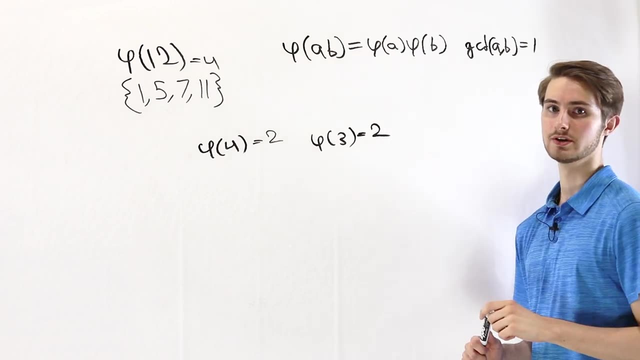 than or equal to 12, which are co-prime to 12.. And since there are four elements in this set, 5,- 12 equals 4.. Now we're going to take a look at the right side of the equation. 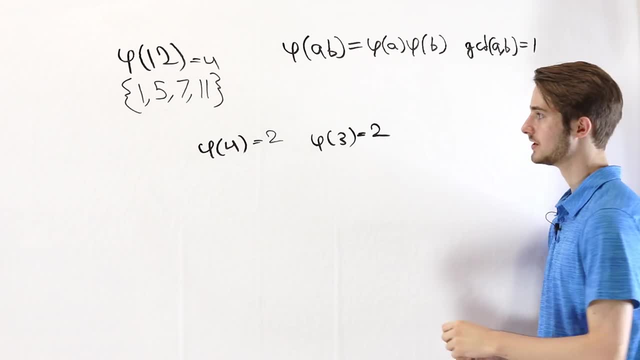 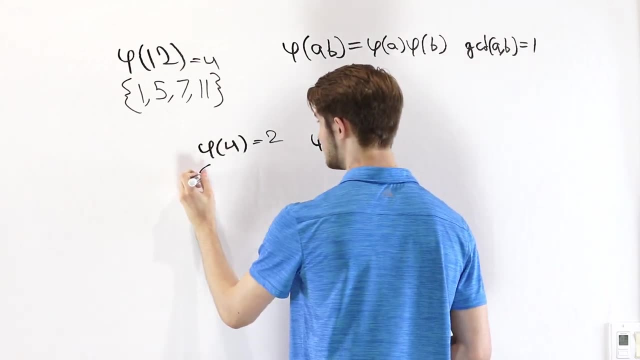 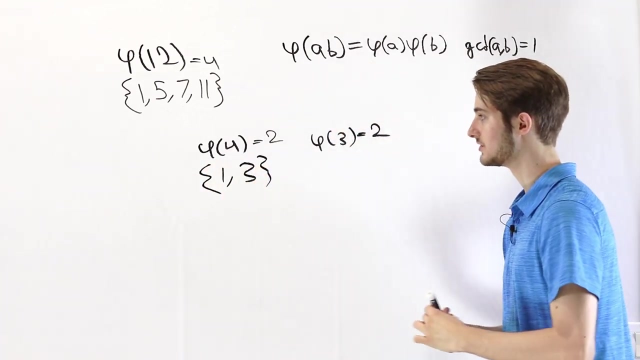 Let's start by considering the sets of numbers that are co-prime to 4, and then co-prime to 3.. Like we saw before, the set of numbers that are co-prime to 4 and less than or equal to 4,, that's going to be 1 and 3, because these are the numbers that don't 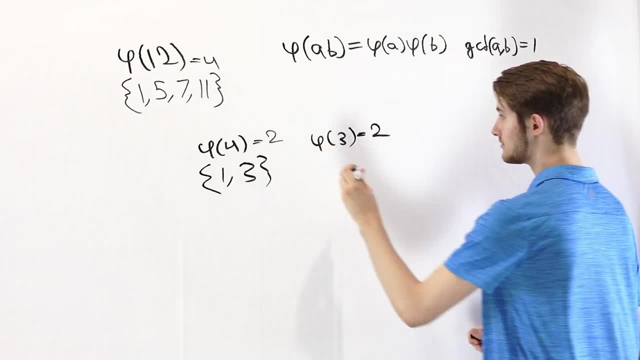 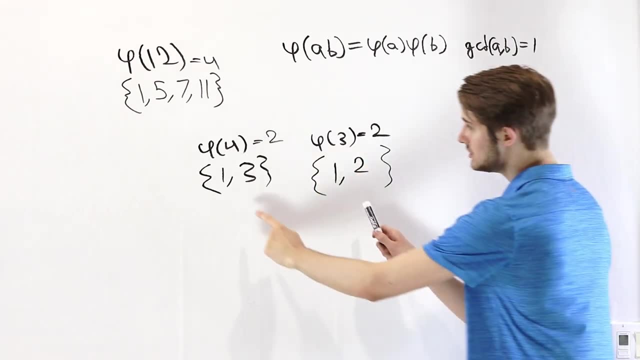 have any factors of 2.. Over here, when we're looking at 5, 3,, the numbers co-prime to 3 are 1 and 2.. We're going to take these two sets and combine them by turning them into ordered pairs. 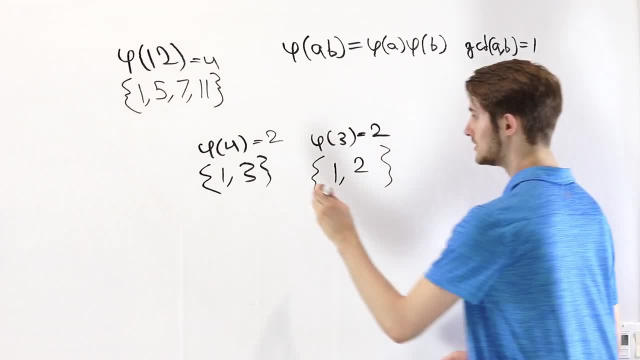 If you're familiar with the set of numbers, you'll know that the set of numbers that are co-prime to 3 is a set of numbers that are co-prime to 3.. If you're familiar with set theory, we're doing a Cartesian product which looks like this, but you don't need to know that. 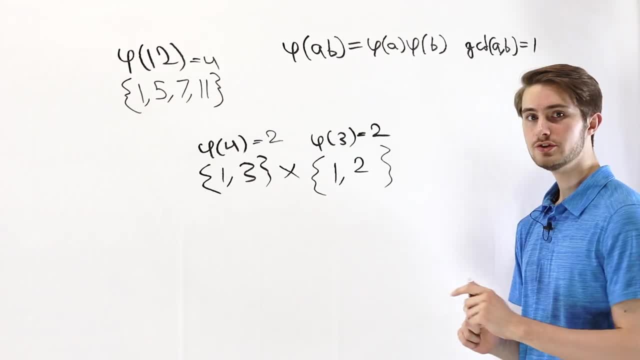 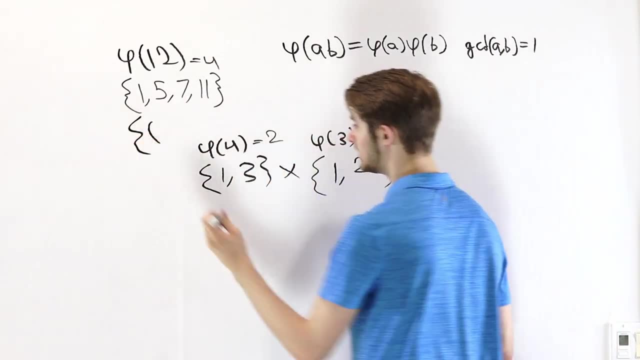 to understand what's going on here. So again, we're going to construct a new set that has ordered pairs in it, And the way that we'll do that is we'll take the first number in the ordered pair from the first set. For example, we could use this 1. And then we're going to take the. 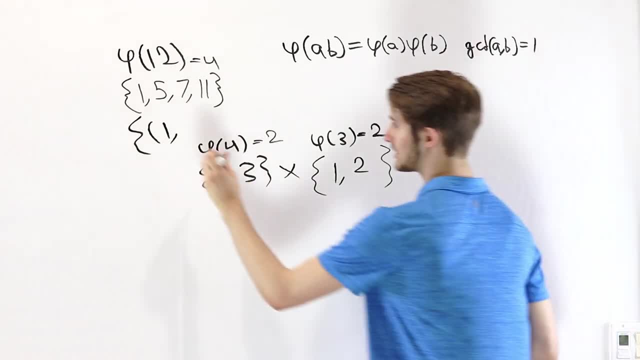 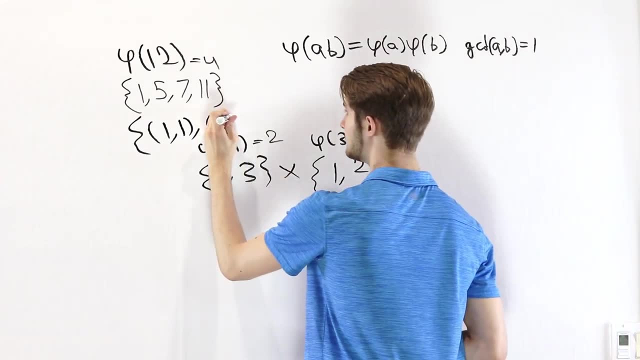 second number in the ordered pair from this set. For example, it could be again a 1.. We could also have a 1 from the first set and a 2 from the second set. We could also have a 3 from the first set and a 1 from the second set. 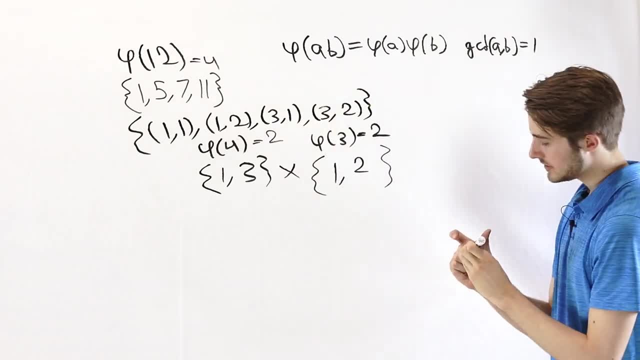 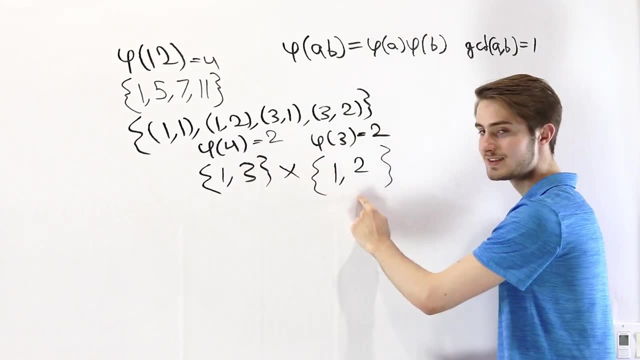 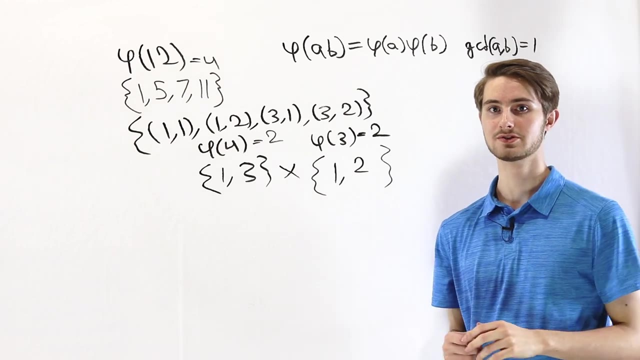 or a 3 and a 2.. So this set right here gives us all of the ordered pairs, with the first number from the first set and the second number from the second set. Notice that this set right here has four elements, And the reason for that is that each of these sets has 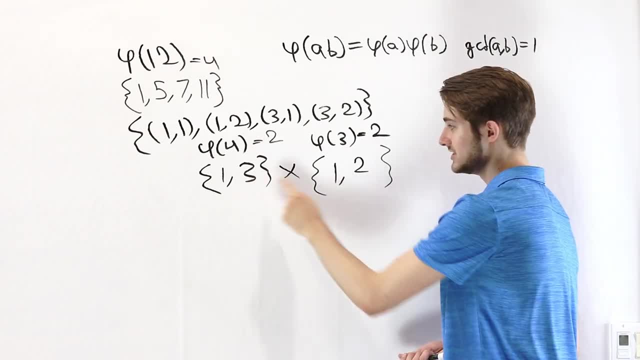 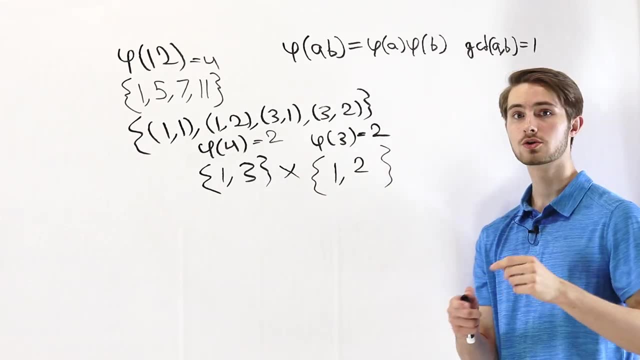 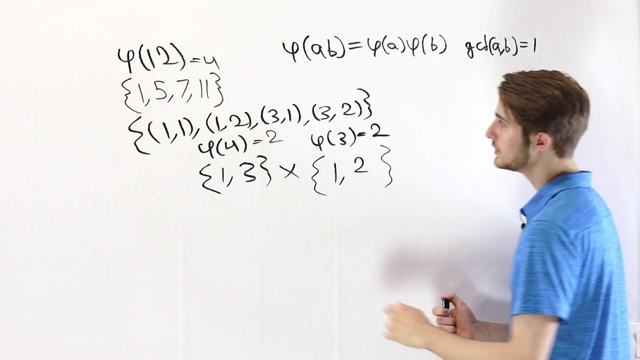 two. So, because we're looking at picking a number from each of these sets, there are two ways to pick from this set and two ways to pick from this set. So the total number of pairs is 2 times 2, 5a times phi of b. So if we can show that for any given number, ab. 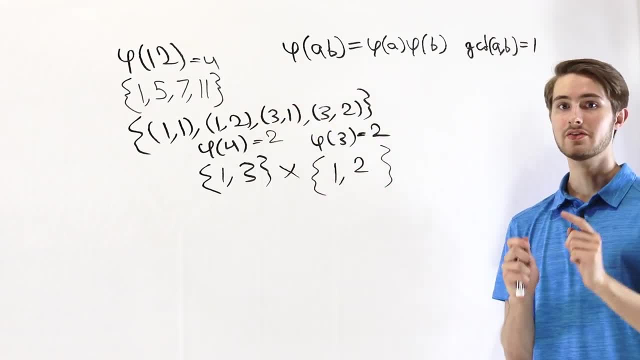 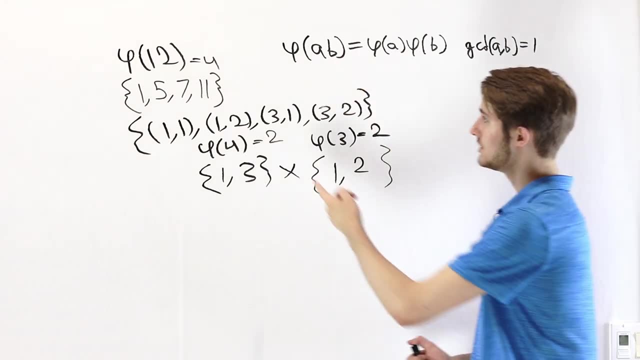 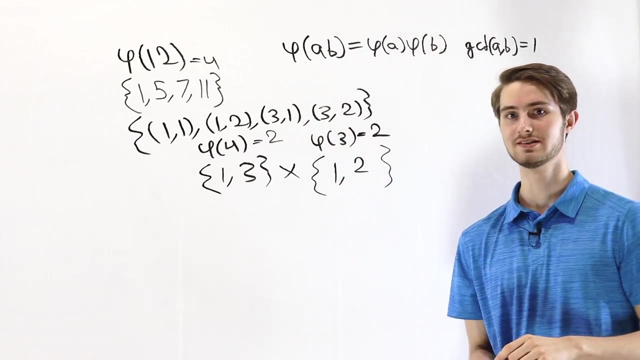 these two sets have the same number of elements. that proves that 5ab equals 5a times 5b. Of course, in the case with ab equal to 12, it's pretty obvious that we have four elements in the first set and four elements in the second set. But how are we going to prove that? for a general case, 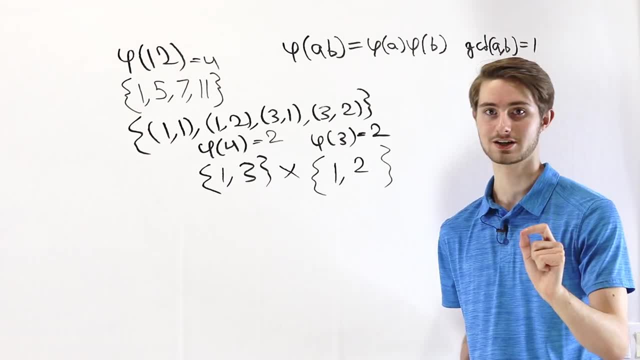 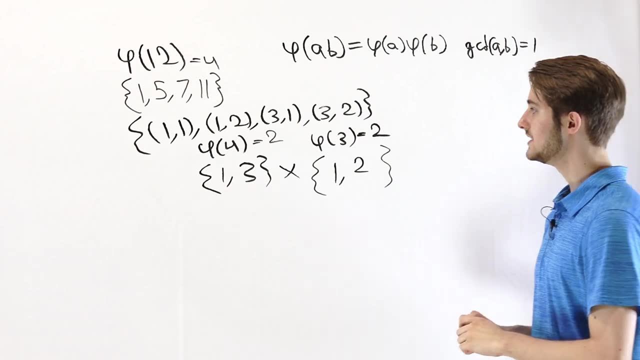 In order to do that, we're going to use something called a bijective function. Now, if you aren't familiar with how this works, I have a video on bijections in the description. The idea is that if we have two different sets here, 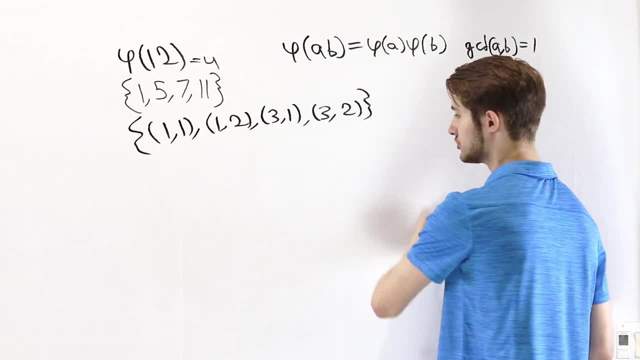 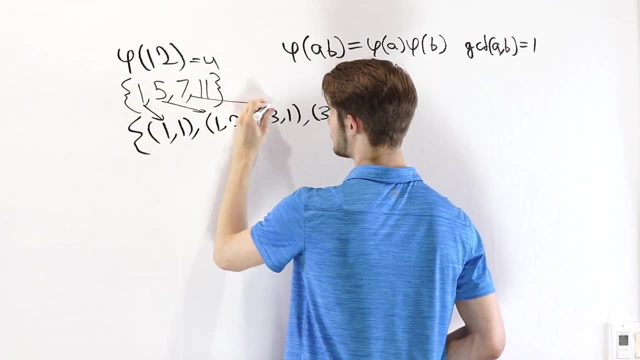 if we can construct a bijective function, we're going to have a bijective function. A bijective function is a bijection between the two sets, meaning we have an exact one-to-one correspondence where we can map each element in the first set to one element in the second set. 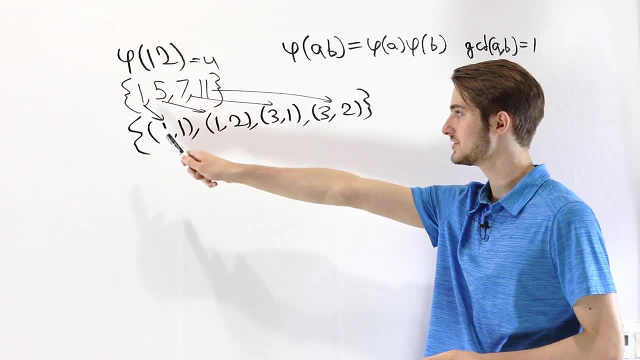 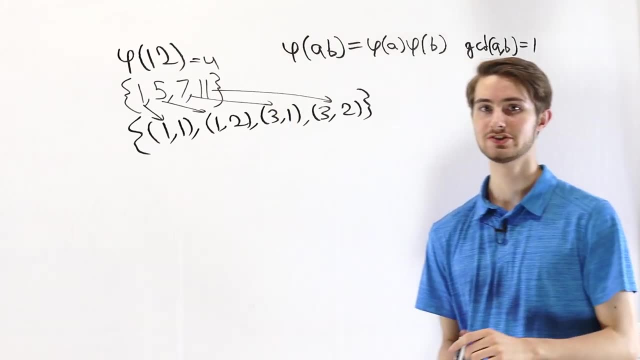 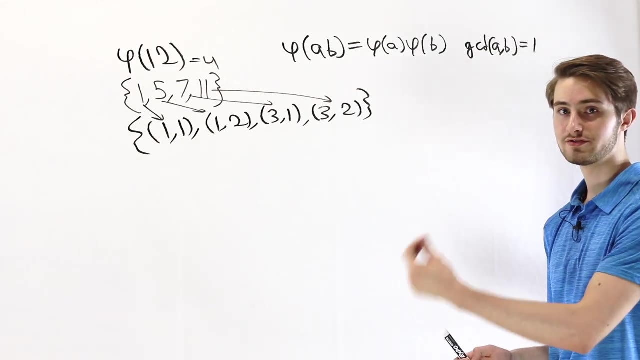 like this: And there's one element for the first set for every one element in the second set. This proves that there are the same number of elements in each set. Again, you can check the video in the description where I explain how this works. So we want to try to find. 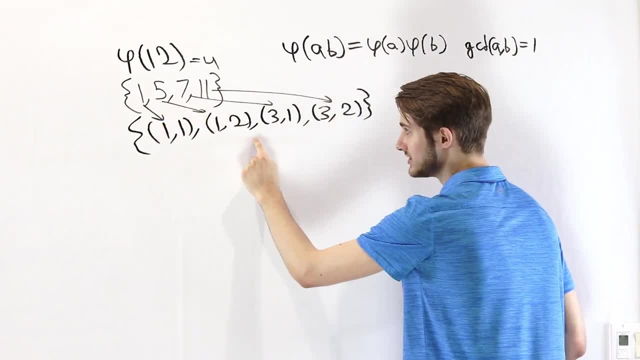 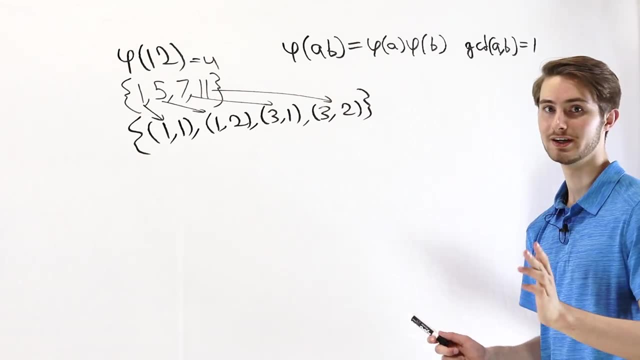 a bijective function in the first set. So we're going to try to find a bijective function in the way to go from this first set to this second set. that is a bijection. If we can find some function that does that, then we're done. We've proved this theorem. Now I'm going to pick a function. 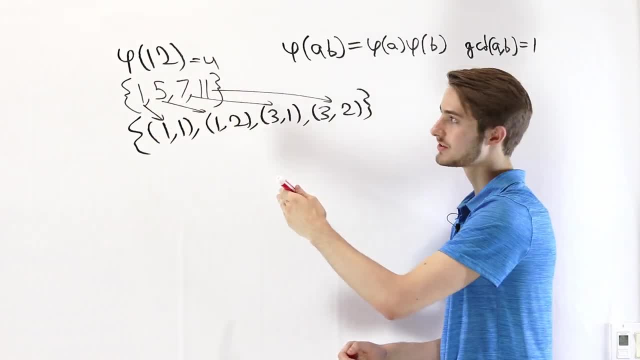 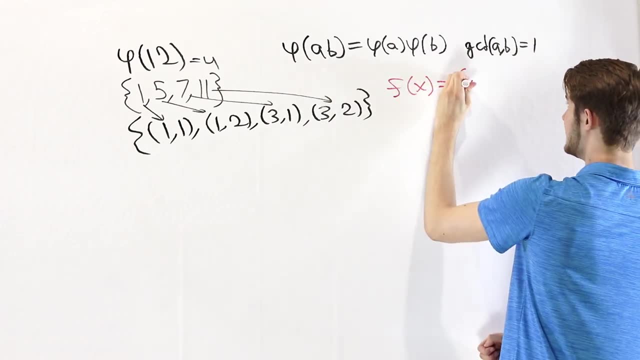 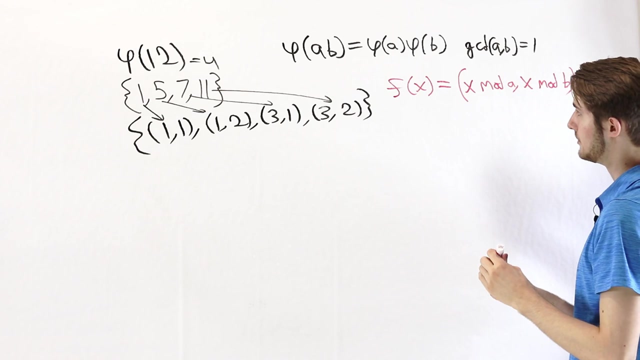 that looks like this For any element x, that's in the first set. we're going to take f of x to be the ordered pair: x mod a, comma, x mod b. Now, this is an ordered pair where each number is x reduced mod one of the numbers a or. 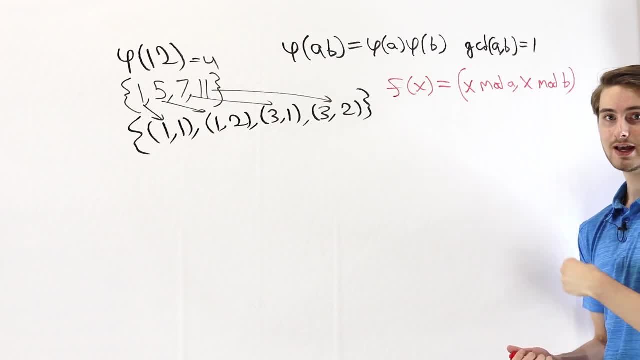 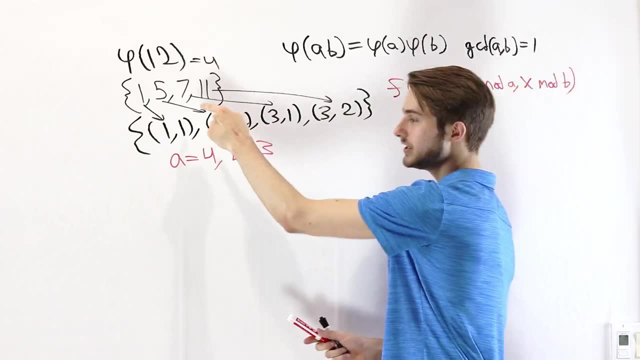 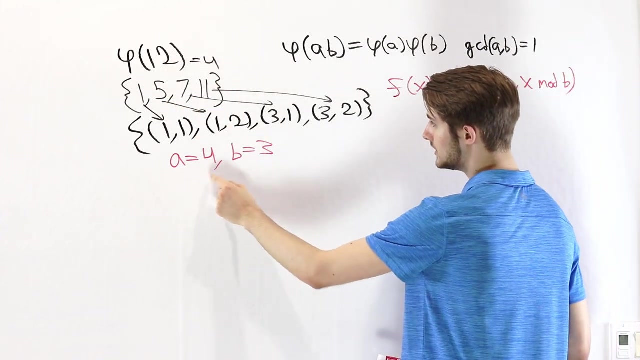 b. If you aren't familiar with reducing numbers, mod n- I have a video on that in the description as well. Let's take a look at how this function works using the example that we have right here. We're looking at 5,, 12, and in this case we're taking a equal to 4 and b equal to 3.. 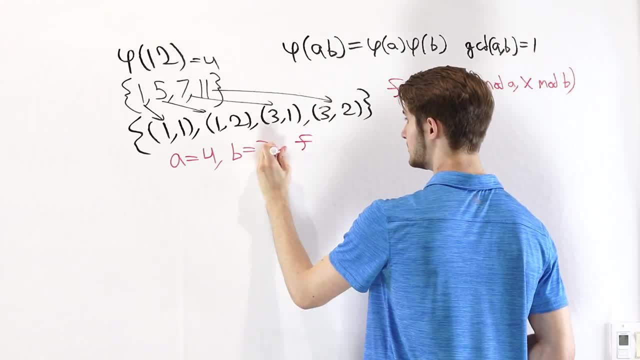 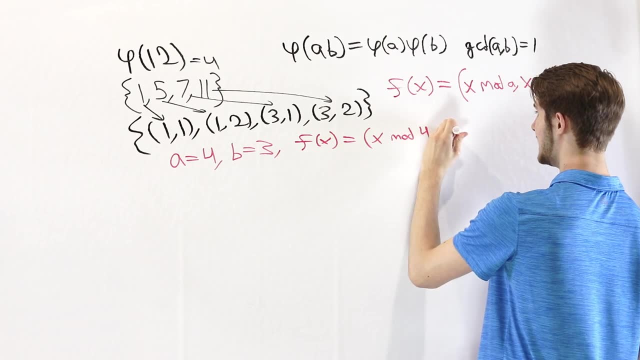 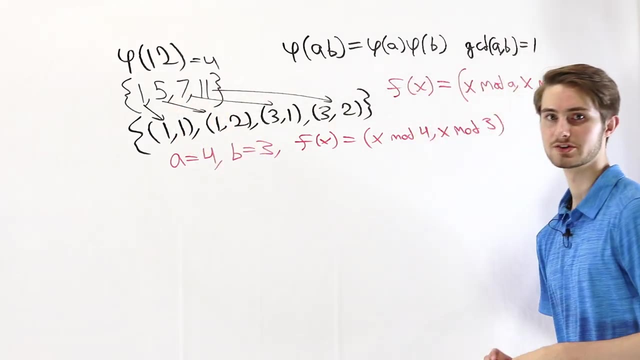 So that means that our function here is going to be: f of x is equal to x mod 4, since a is 4 and then x mod 3.. So let's see how that works for the four numbers that we have in our set. First, 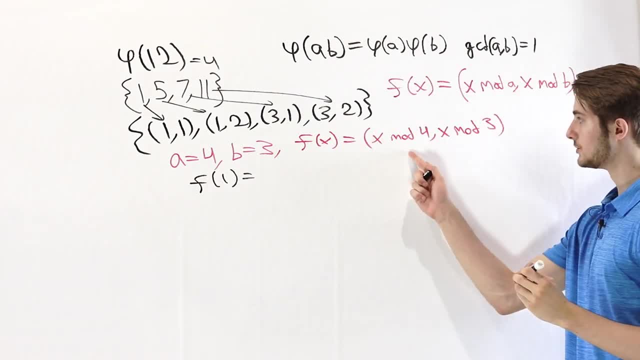 we're going to look at f of 1. That's going to be 1 mod 4, 1 mod 3.. Well, 1 mod 4 is 1 and 1 mod 3 is 1.. So that's simple enough. 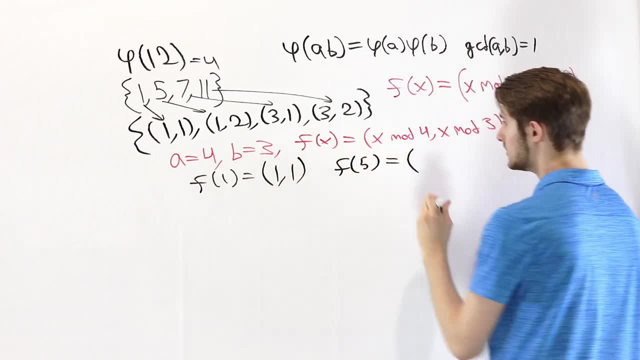 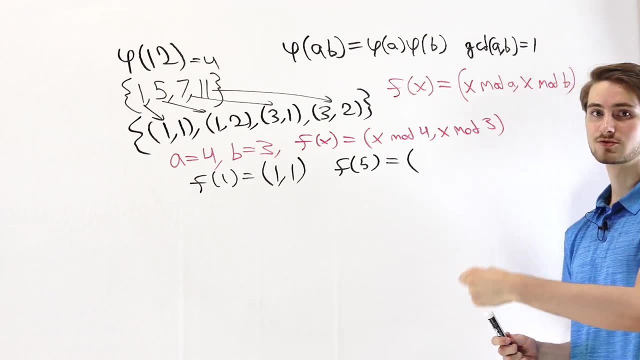 Next we have f of 5.. What is 5 mod 4?? Well, we can reduce 5 mod 4.. If we subtract 4, we get 5 minus 4 is 1.. So 5 mod 4 is 1.. Similarly, with 5 mod 3, we subtract 3.. So we get 5 minus 3 is 2.. 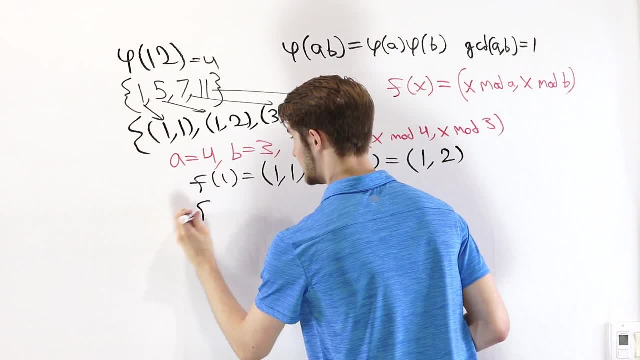 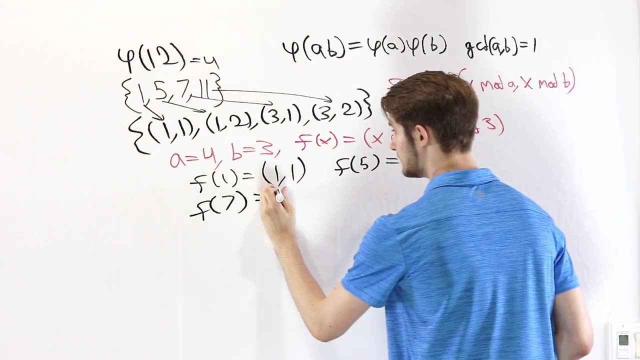 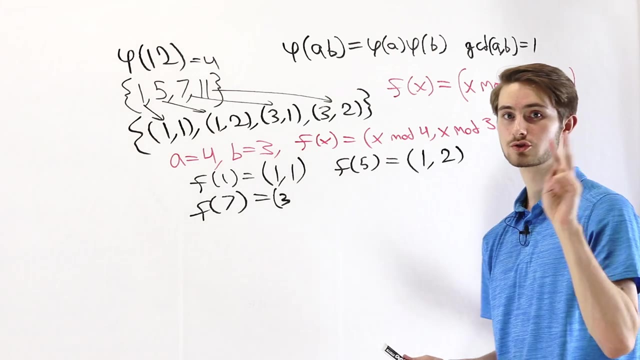 So our ordered pair is 1, 2.. Next, f of 7.. What is 7 mod 4?? Well, if we subtract 4, we get 3.. So 7 mod 4 is 3.. Next, 7 mod 3. Notice that 3 actually goes into 7 twice, So we. 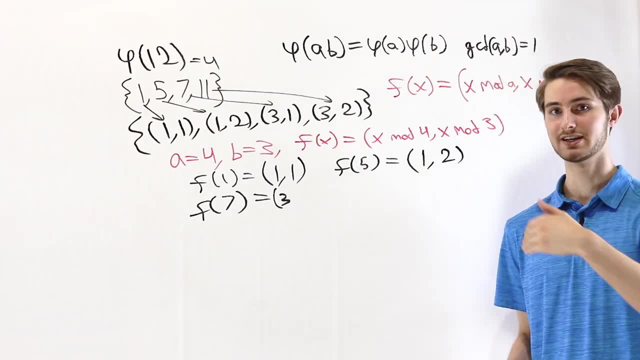 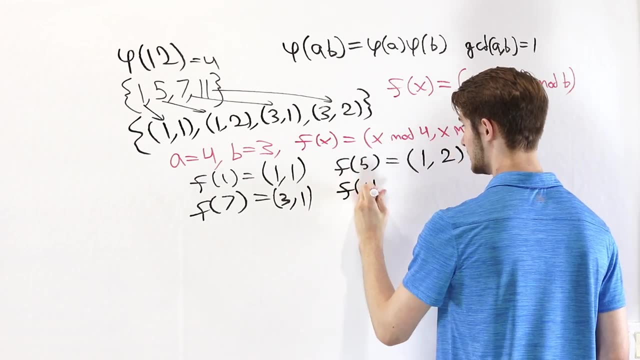 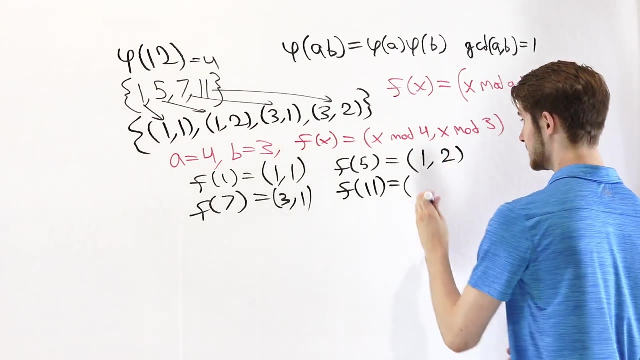 can subtract 3 twice, That's going to be 7 minus 6, which is 1.. So 7 mod 3 is 1.. And finally, f of 11.. What do we get here? With 11 mod 4, we can subtract 8, and that's going to give us 3 as the 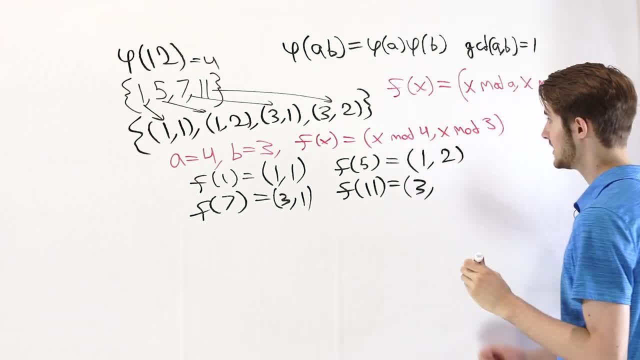 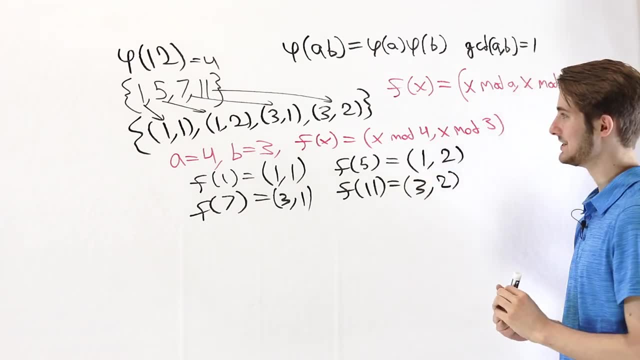 remainder. So 11 mod 4 is 3.. And finally, 11 mod 3, we can subtract 9, and we get 2.. This is very interesting because notice that the elements that we get here, these four outputs, 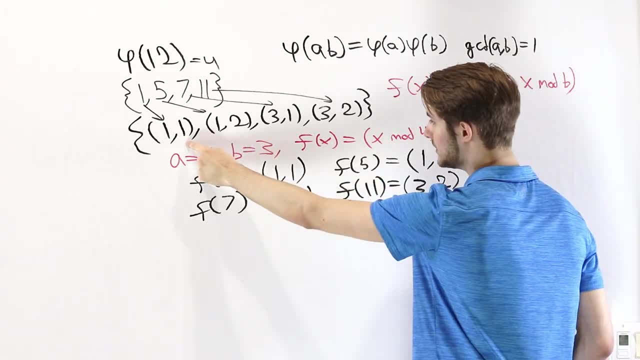 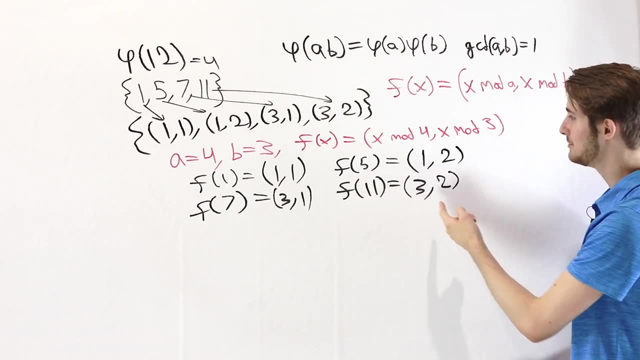 these are exactly what we see in our set: 1, 1, 1, 2, 3, 1, 3, 2.. How does that work? How did we get these outputs in such a nice order with this function? 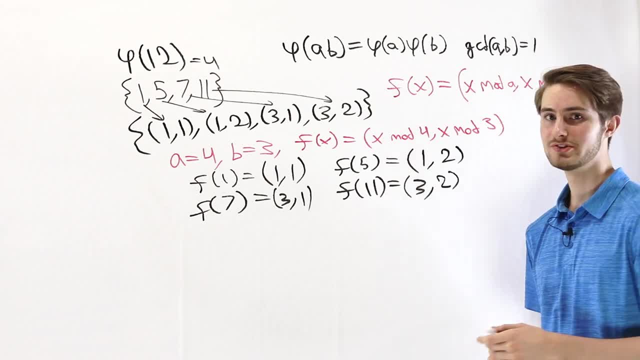 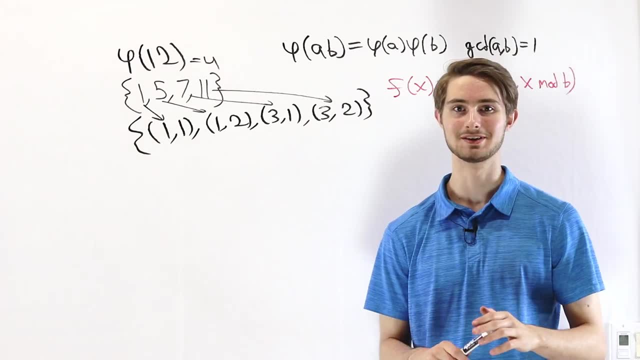 Why do we get these outputs in such a nice order? Why do we get these outputs in such a nice order? Why do we get the exact values from those sets with phi of 4 and phi of 3?? In order to understand how this works and where the Chinese remainder theorem comes in. 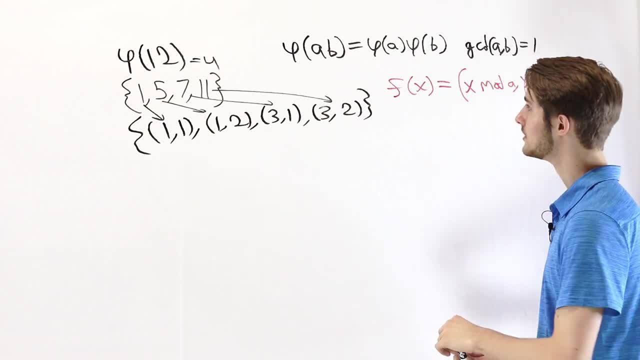 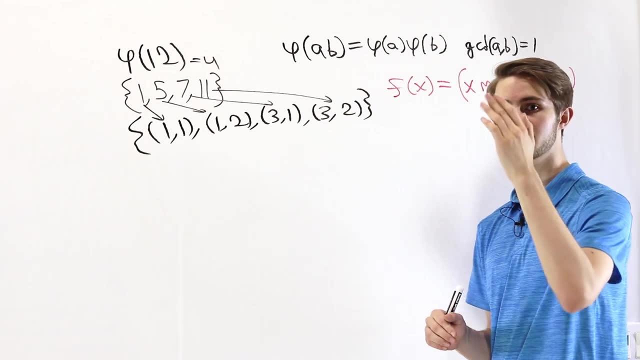 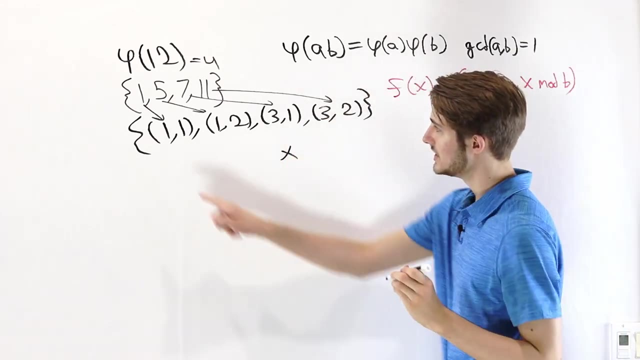 we're going to take a look at coprime numbers. Remember that this first set is related to phi of ab and that's talking about all of the numbers between 1 and ab that are coprime to ab. So for any number- x- that's in this first set. 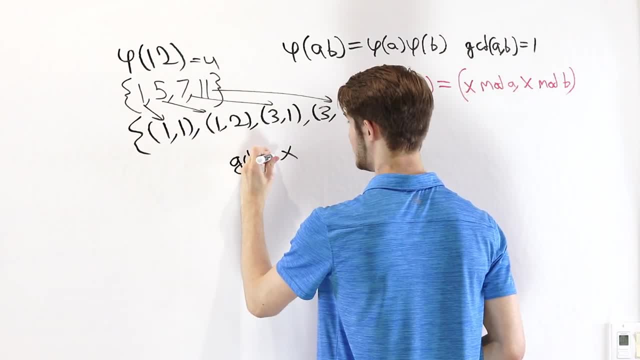 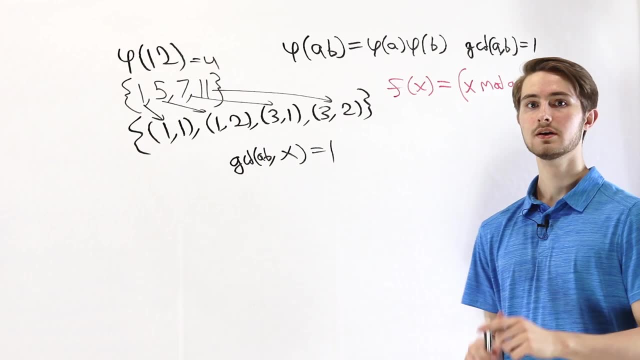 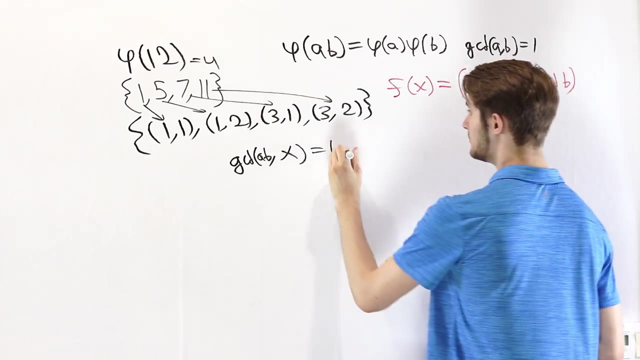 we know that it must be co-prime to a- b by definition, meaning the greatest common divisor of a, b and x is equal to one. one of the properties of co-prime numbers is that if a, b is co-prime to x, then we know that a and b are both also co-prime to x. 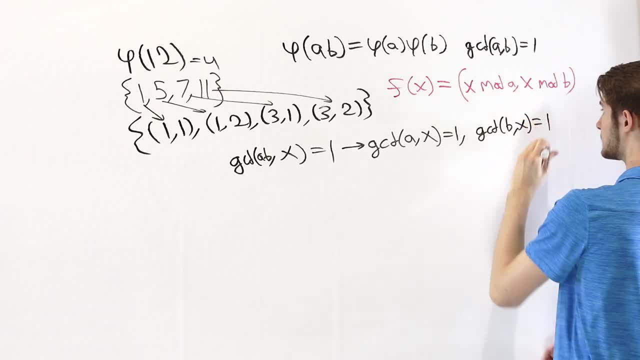 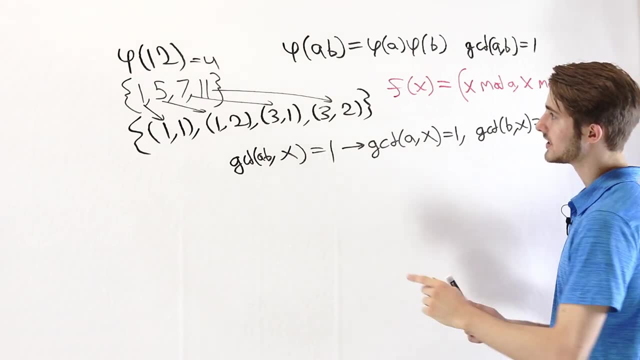 again. this is in my video on co-prime numbers. you can check the link in the description for that. so because in this first set all the numbers are co-prime to a- b, we know that all the numbers are also co-prime to a and b. and the important property, which is something i talk about in 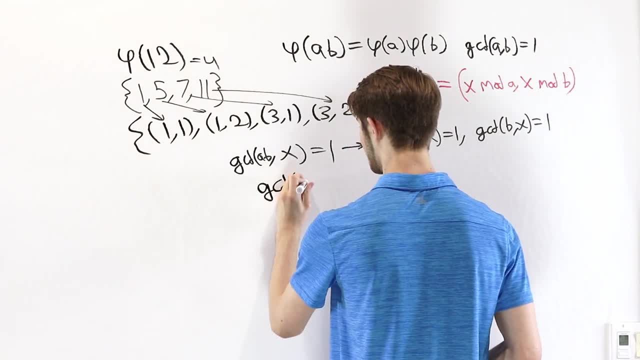 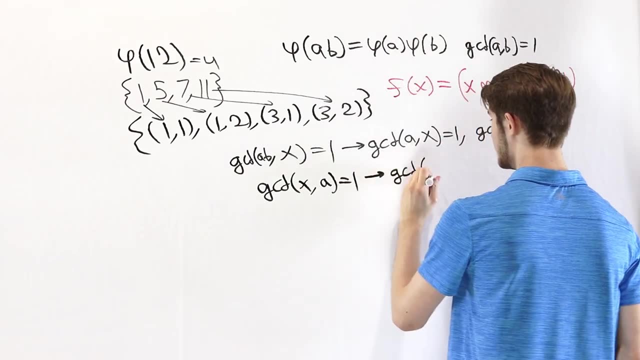 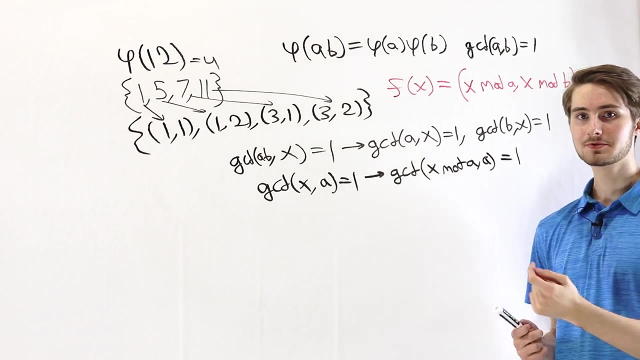 that video. in the description is that if x is co-prime to a, so if the greatest common divisor of x and a is one, then we know that when we reduce x mod a it will still be co-prime to a, and that comes from the fact that reducing x mod a just involves adding or subtracting. 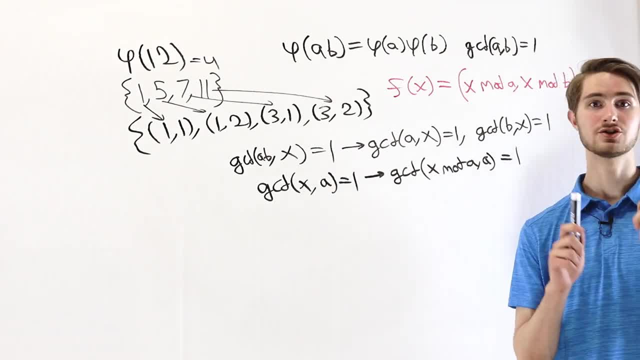 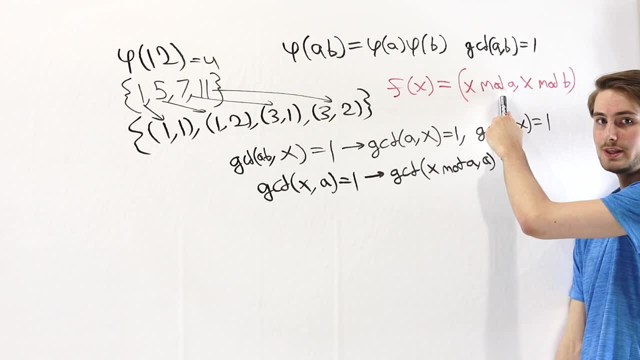 multiples of a, and when we do that, it doesn't change whether the number is co-prime to a. so we know that x mod a- this first number in the pair, is co-prime to a. and similarly, if we reduce x mod a to a, we know that x mod a is co-prime to a. 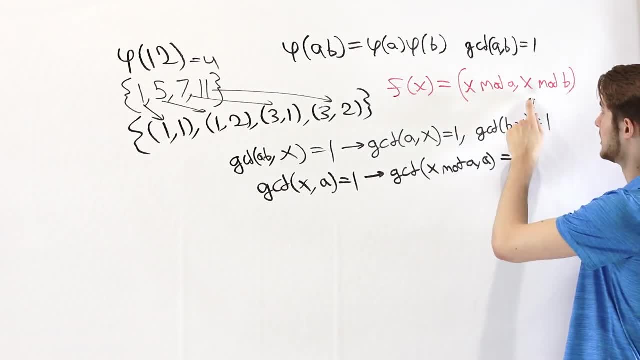 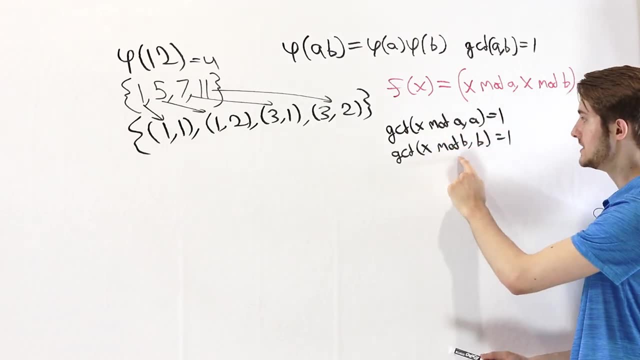 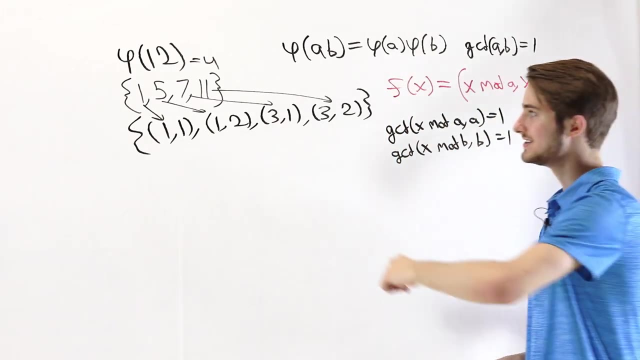 similarly, we know that x mod b is co-prime to b. now, the reason it's important that x mod a is co-prime to a and x mod b is co-prime to b comes down to the way that we constructed these sets over here. remember that this second set is the set of all ordered pairs, where the first number 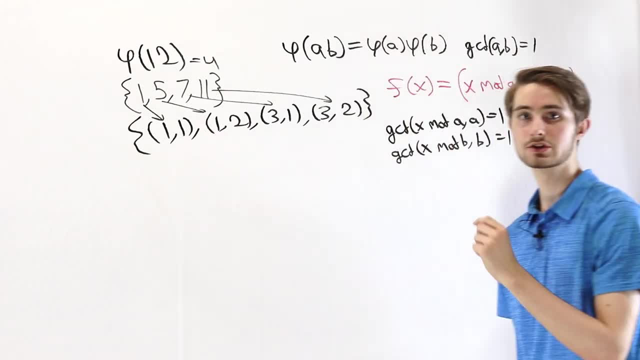 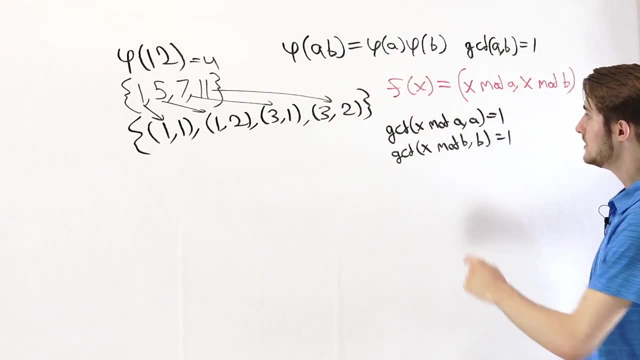 is co-prime to a and the second number is co-prime to b. that's why the number of elements in the pair is co-prime to a and the second number is co-prime to b, and the second number there is 5a times 5b. so if x mod a is co-prime to a and x mod b is co-prime to b, what that's telling us? 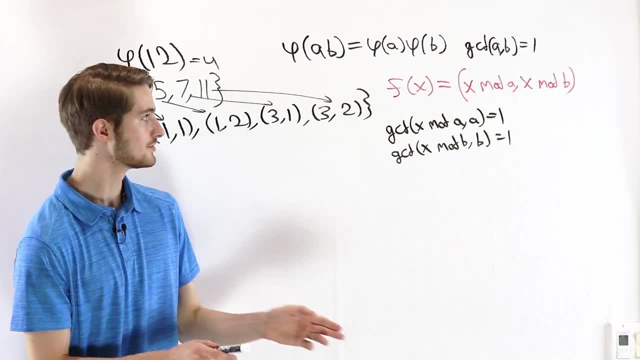 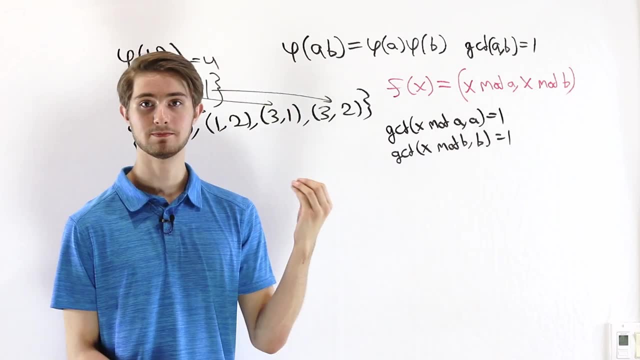 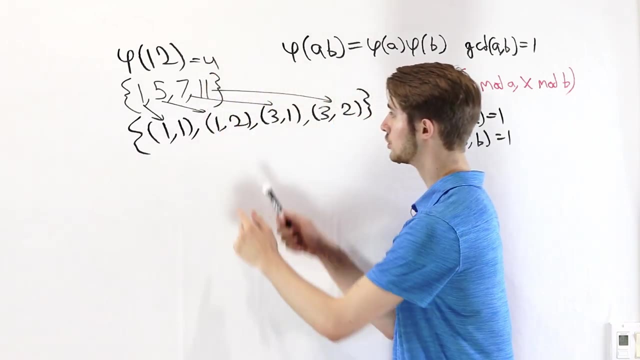 is that this ordered pair gives us a pair of numbers where the first number is co-prime to a and the second number is co-prime to b. since we reduced them mod a and mod b, they're also between 1 and a or b and therefore they're going to be in this second set. 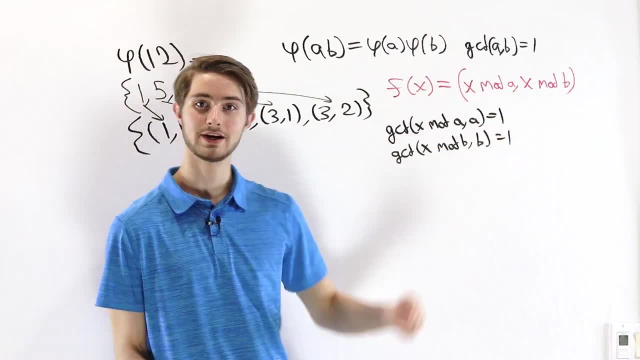 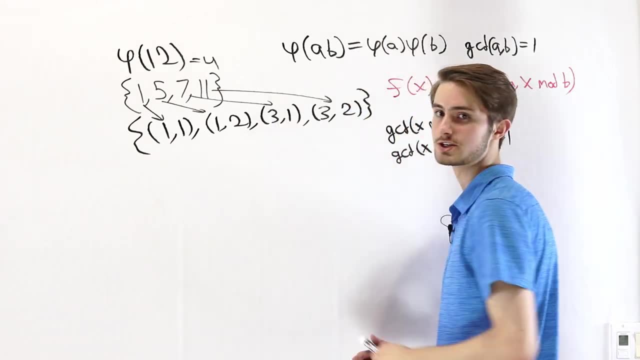 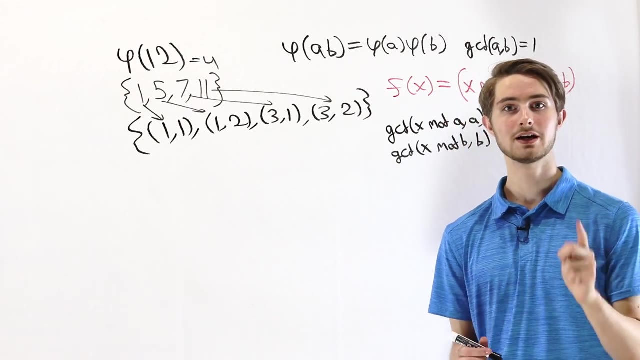 that's telling us that this function always gives us an ordered pair that's in the second set, and that's a very important first step to proving there's a bijection between these sets. so we've proved that this function goes from the first set to the second set. but now we have to prove. 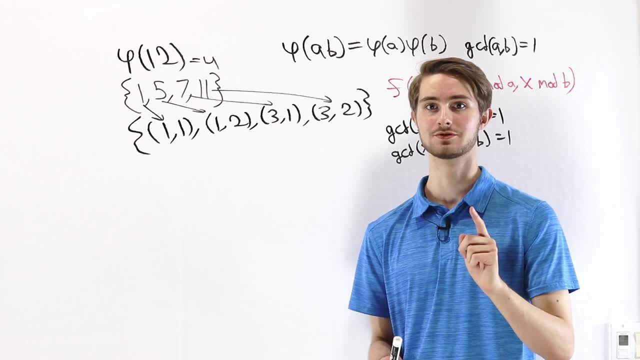 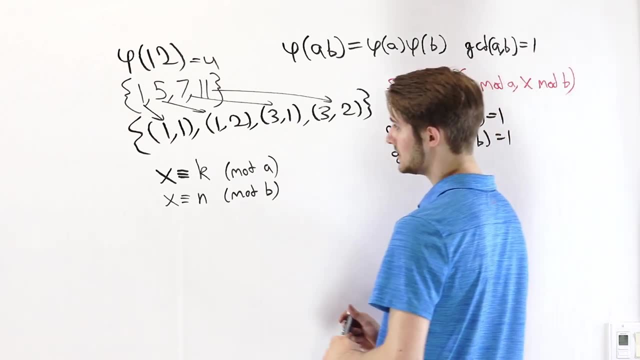 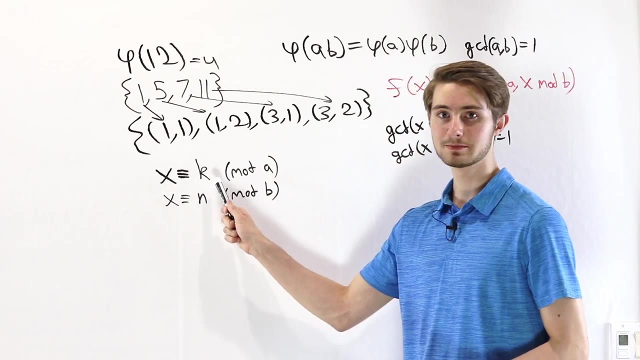 that it's a bijection, and this is where the chinese remainder theorem comes in. so let's talk about what the chinese remainder theorem says. the chinese remainder theorem says that if we have a system of two congruences, where we have x is congruent to some number, k. 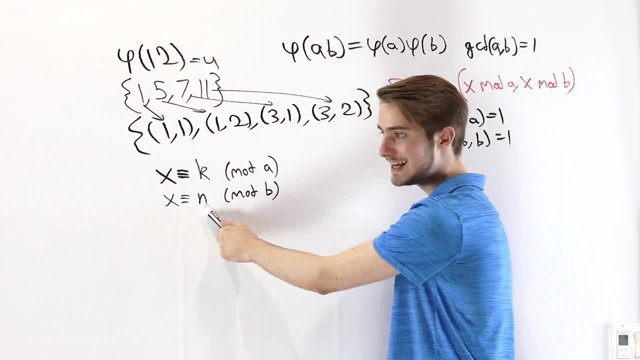 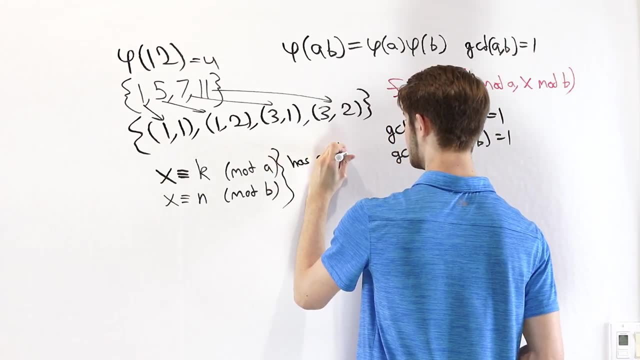 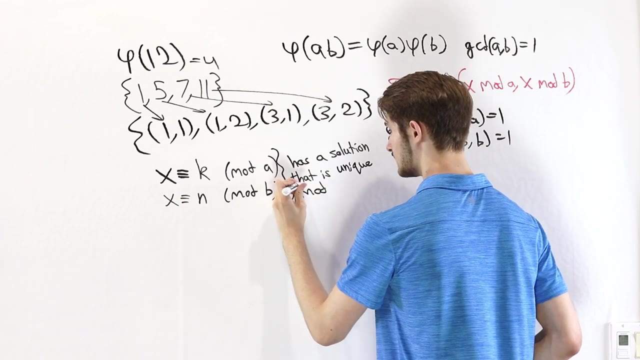 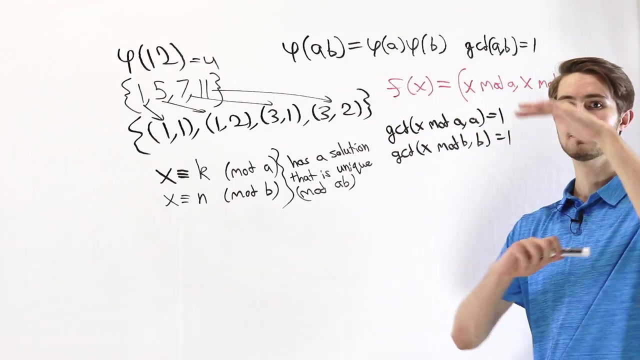 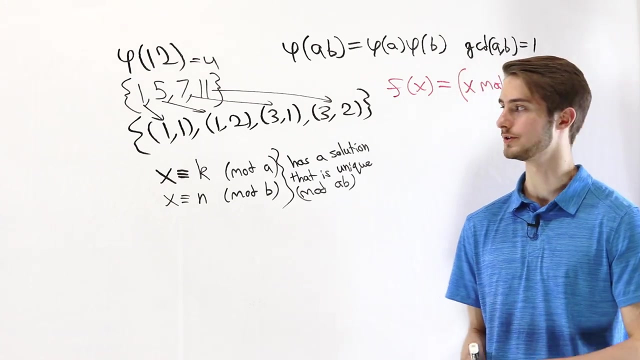 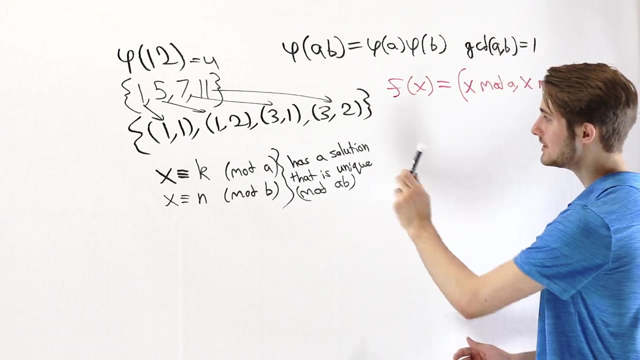 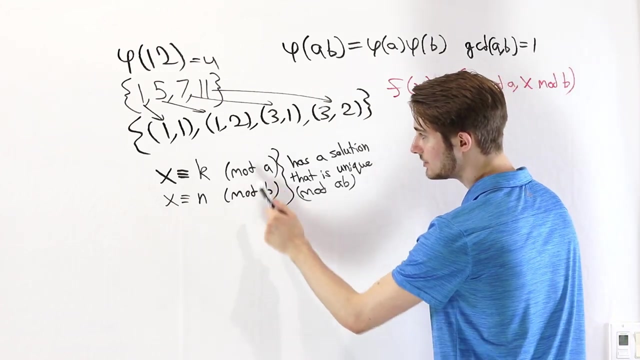 mod a and x is congruent to some number, n mod b. this system of congruences has a solution. and also that the solution is unique: mod a times b. in other words, every solution has vol� must be musical toissements in our system and then naturally in function, we have two congruences. so the useful examples we first use for the chinese remainder theorem. what kinda, basically, what does it lie on taking unconnected congruence and what does it mean how the same q and it's 2 untersähän numbers that we see here in the three given cases fell. or instead, what's uh, instead of what? we're taking this co to the previous possible PREMIUM. 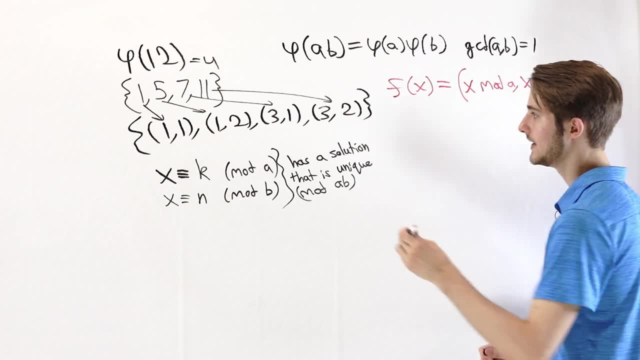 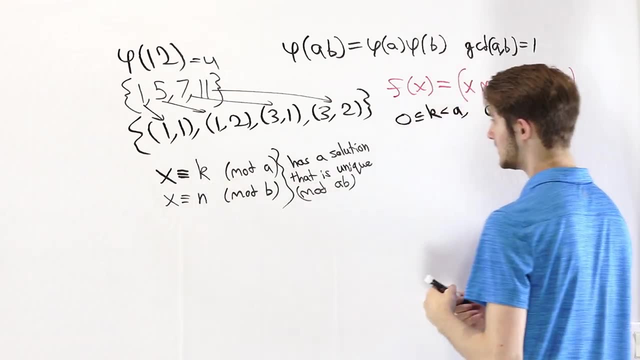 Now the condition for the chinese remainder theorem to be true: If x is congruent to k mod a and we also say that k is between 0 and a, then we can write x congruent to k mod a, as x mod a equals k. 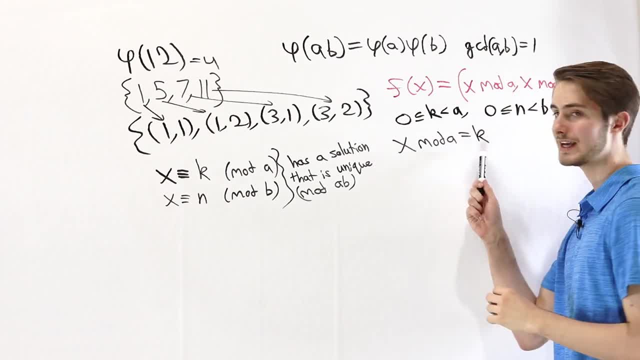 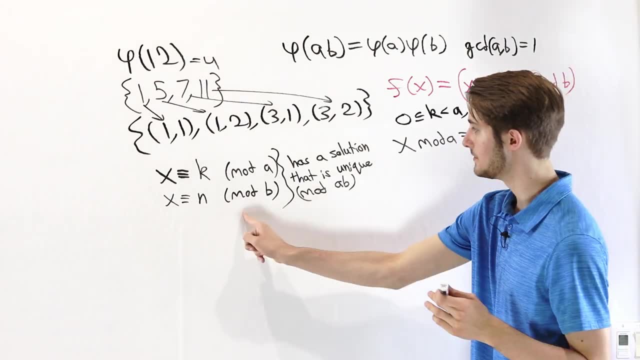 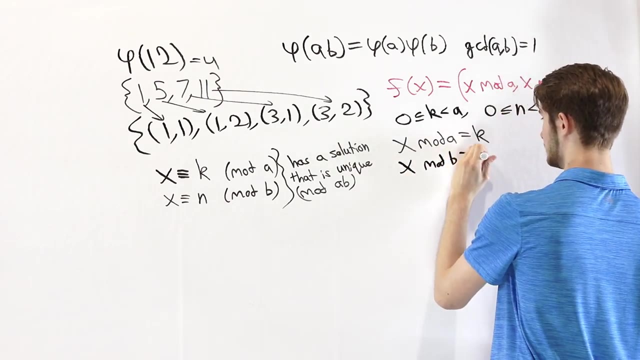 So this is saying that when we reduce x mod a, we get k as our result. We can do the same thing with this second congruence. If x is congruent to n mod b and n is between 0 and b, we can say that x mod b equals n. 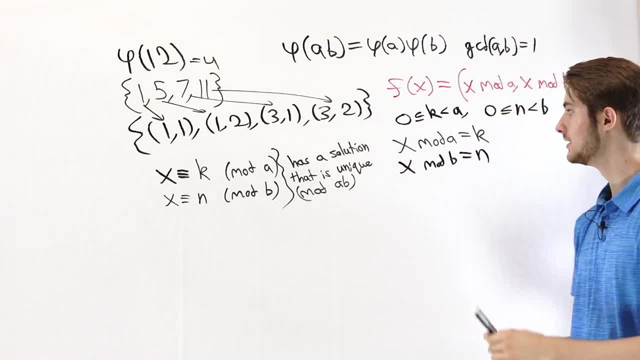 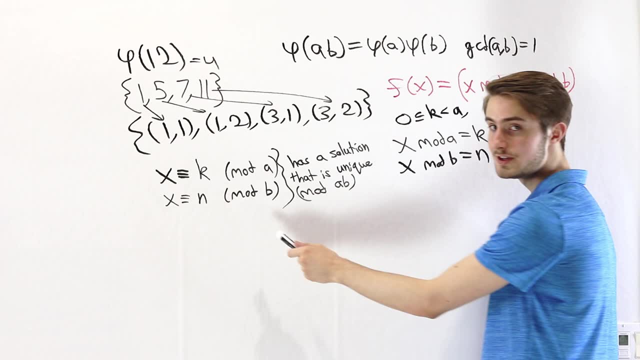 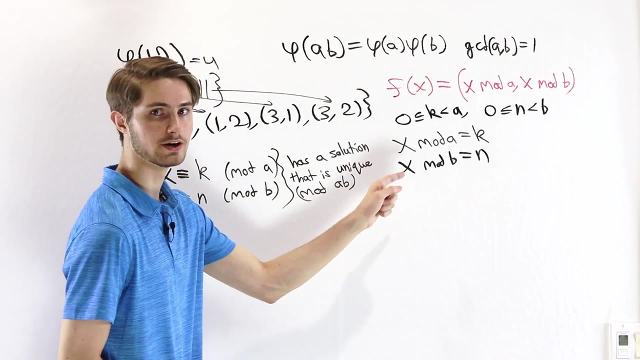 So these two are the same thing. They're both talking about the remainder of x when we divide by b. So the Chinese remainder theorem says that this system of these two congruences has a solution that's unique: mod a- b, Because these two equations over here are equivalent to this system of congruences. 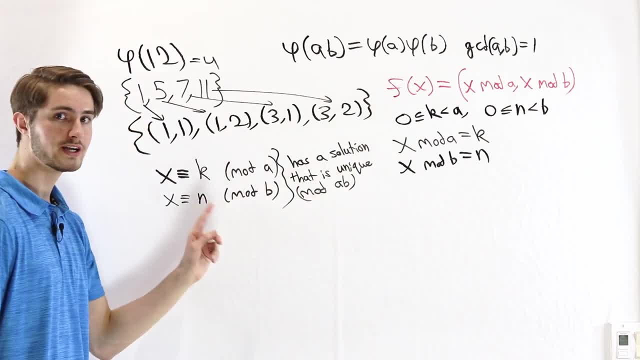 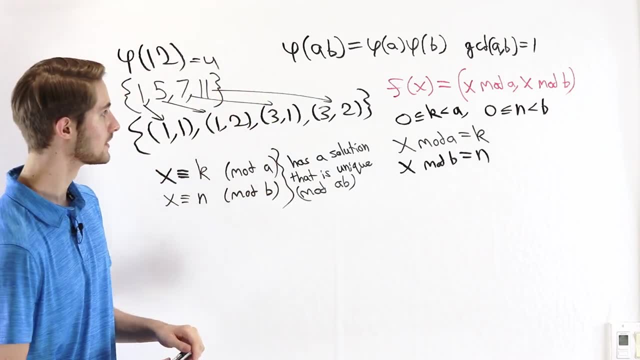 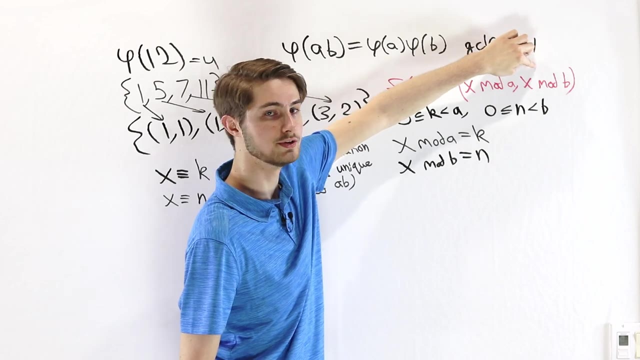 they're describing the same thing By the Chinese remainder theorem. we know that this system of equations has a solution that's unique: mod a- b. Now notice x mod a and x mod b. Those are the two points, the two numbers, in the ordered pair of our function. 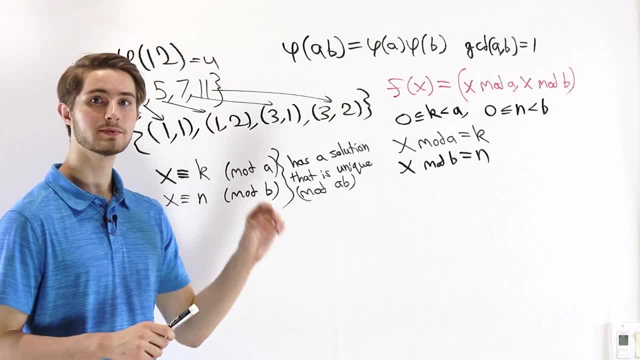 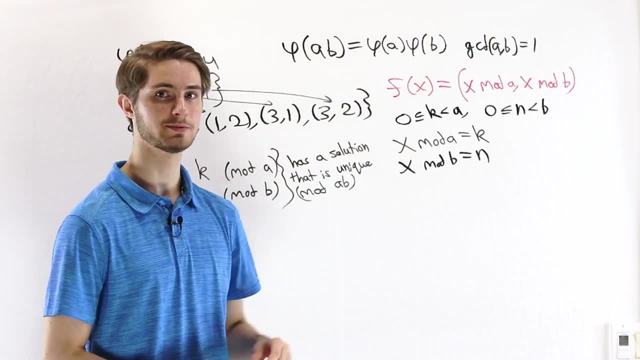 So let's take a step back, remember what we're trying to show and see how we can use this information to determine the congruence To get to that final step. So we just showed that when we're looking at a system of two equations, 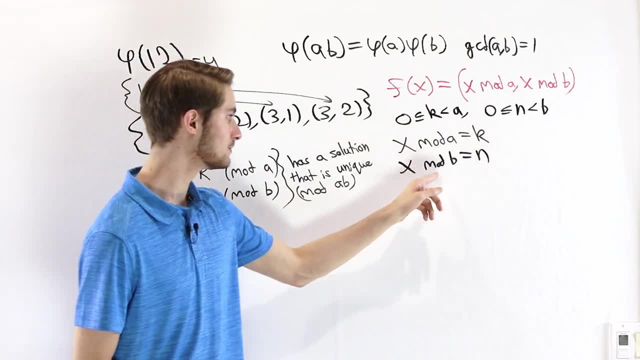 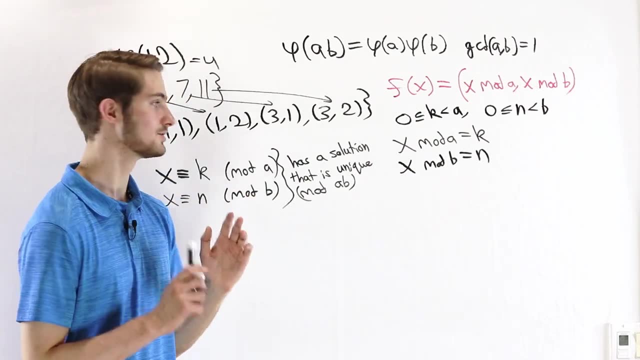 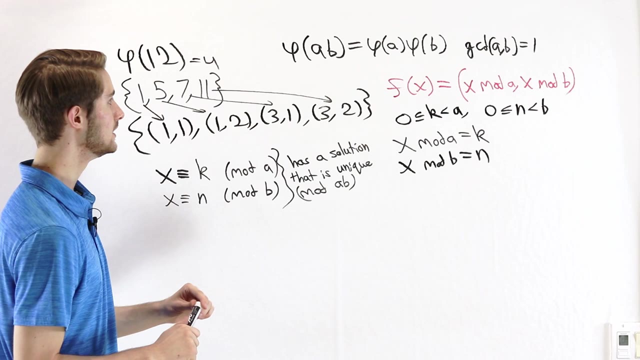 x mod a equals some number k and x mod b equals some number n. there's always going to be a solution, some number x, that satisfies those two equations. Now, our goal when we're trying to prove this totient function identity, is to prove that this function f of x 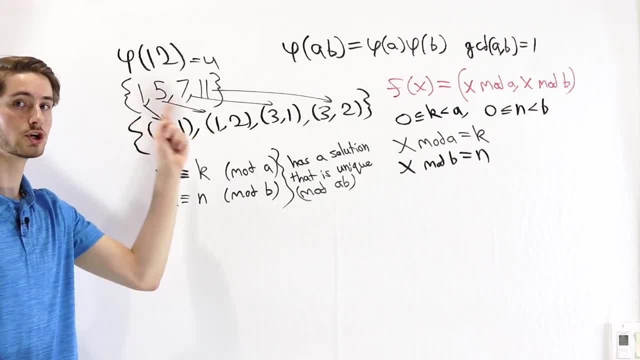 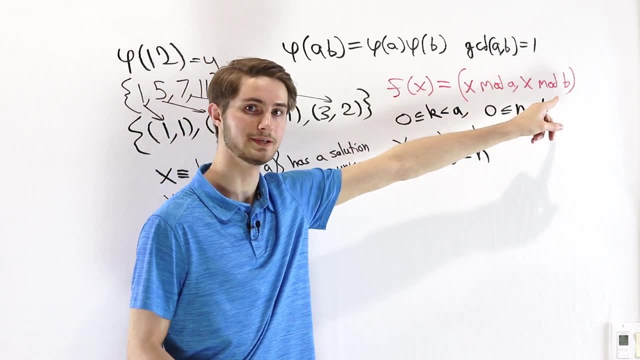 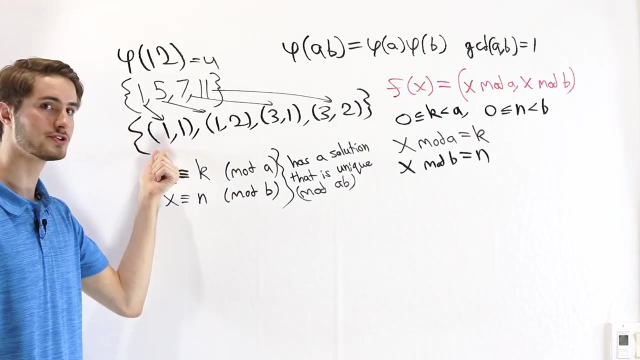 that goes from the set of numbers co-prime to a- b and it goes to x mod a, comma, x mod b. We want to show that that's a bijection with the set of numbers where the first number is co-prime to a. 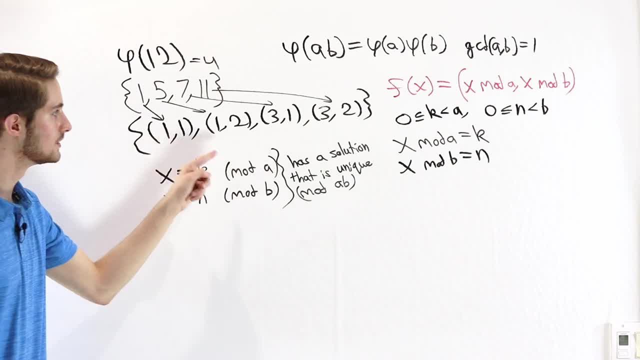 and the second number is co-prime to b. So if we're looking at this situation over here, we know that this first number, k, if we want it to be in this set here, k has to be some number that's co-prime to a. 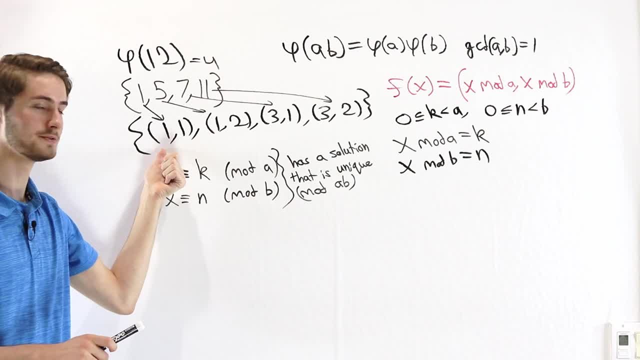 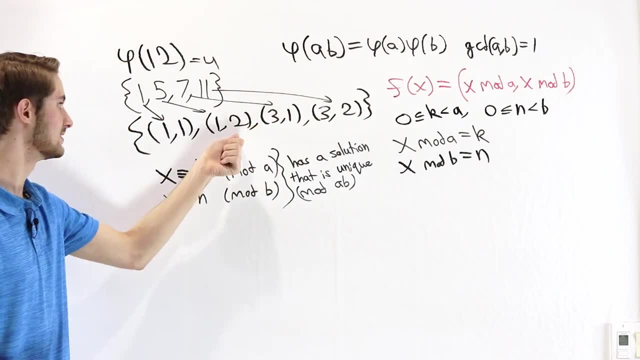 That's going to make it this first point in the set that we want. And similarly, n has to be some number that's co-prime to b, so that it's in this set like the second points here. So let's see what happens if we say: 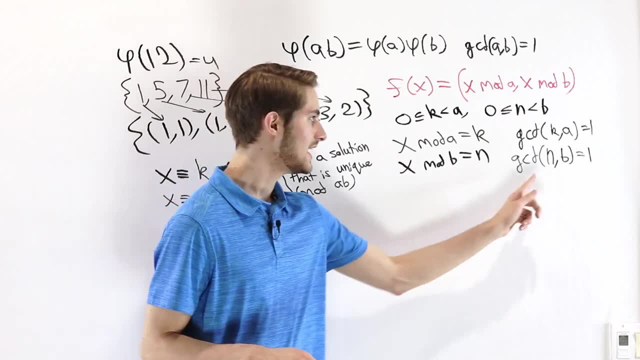 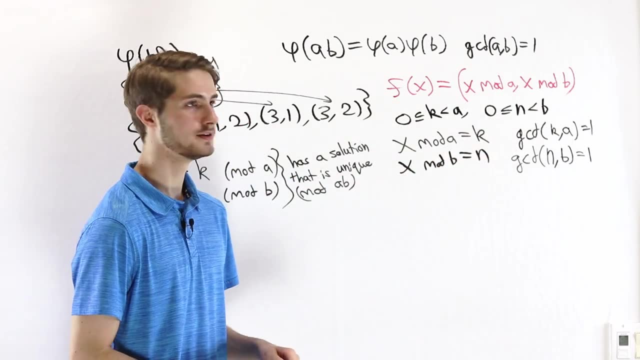 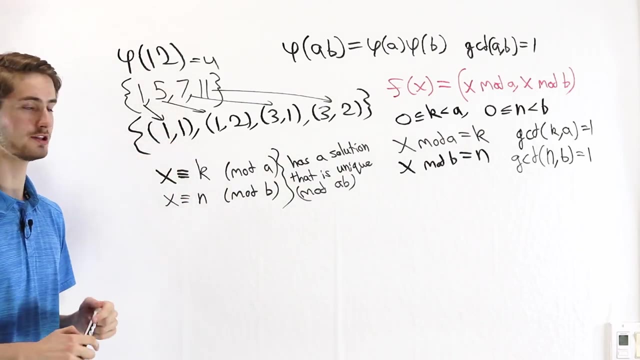 that k is co-prime to a and n is co-prime to b. So if we set these two constraints on the values of k and n, we know that these values- k and n- have to represent some points in the second set that we're looking at here. 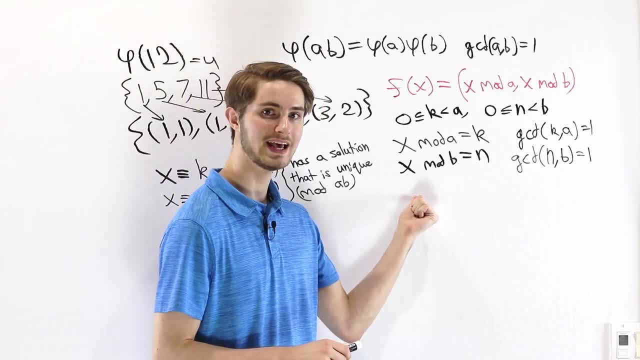 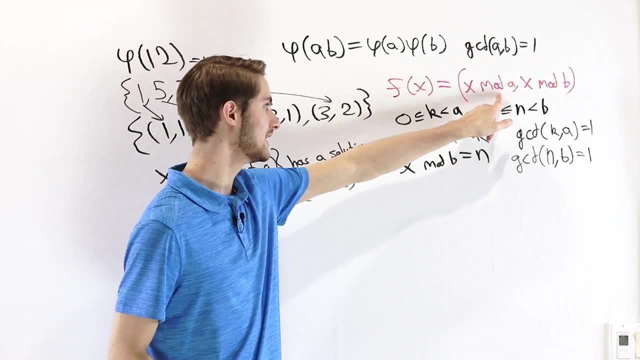 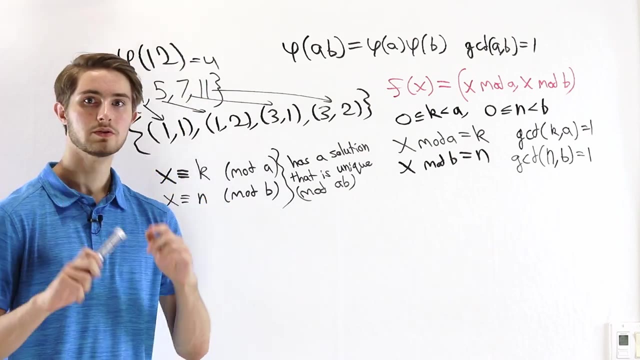 So the Chinese remainder theorem tells us that there's some x that gives the correct point in this second set when we do x mod a and x mod b right here Let's look at some of the properties of that solution. x- Remember that if some number k, 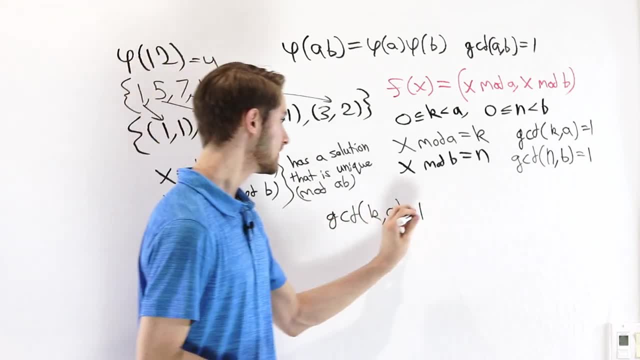 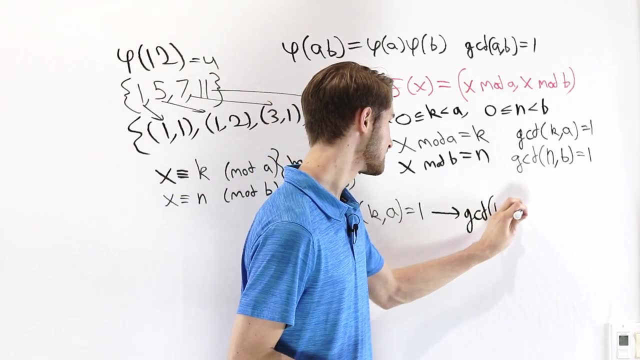 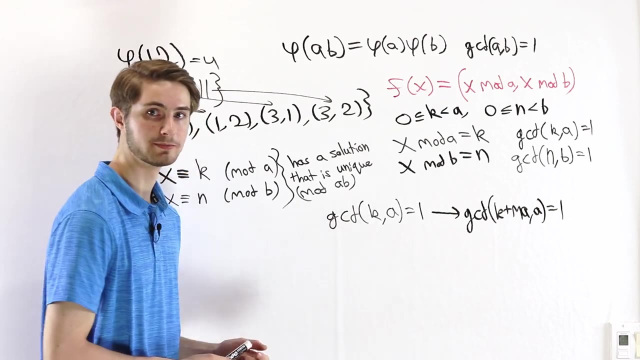 is co-prime to a. one of the results that we can draw from that is that the greatest common divisor of k, plus some multiple of a with a, is also 1. So if we add some multiple of a to the original number, k, 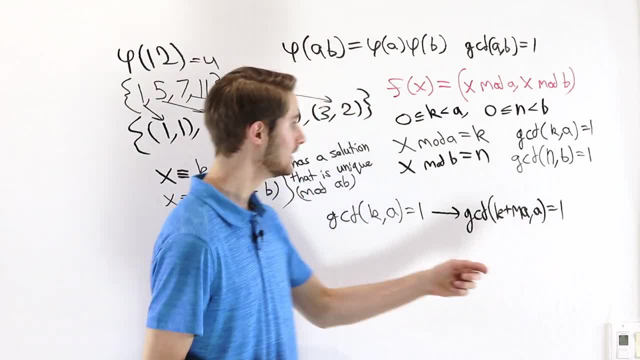 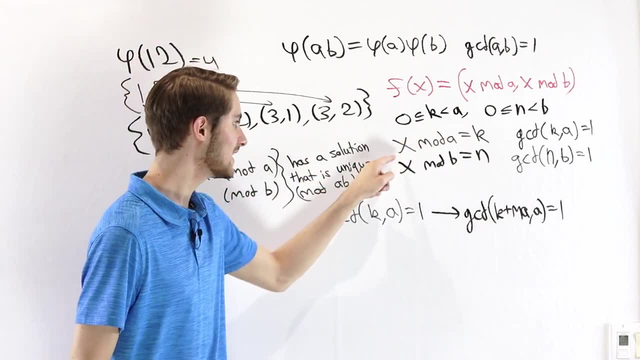 it's still going to be co-prime to a And that's important to what we're looking at here, because we want to look at the properties of a. So we're going to look at the properties of x And k is x mod a. 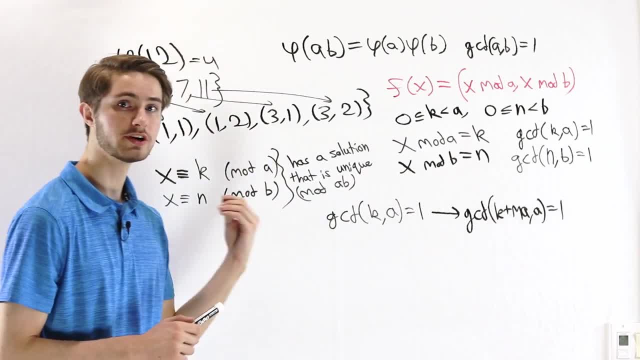 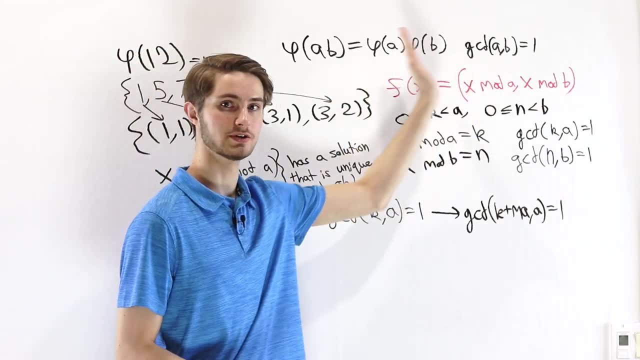 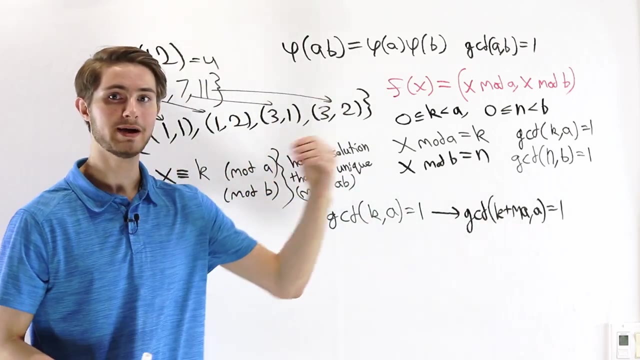 What that means is the way that we get k is by starting with x and adding or subtracting multiples of a until we get a number between 0 and a. That means that the difference between x and k is just a multiple of a. So we can get back to it. 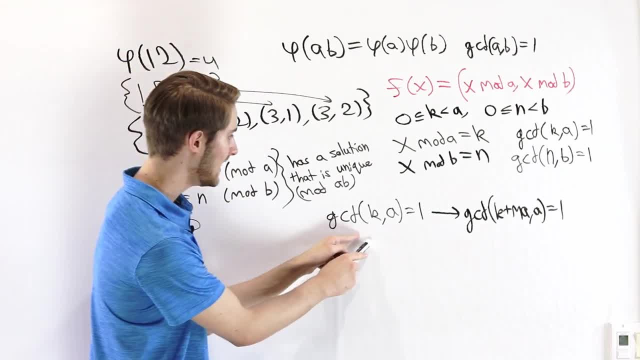 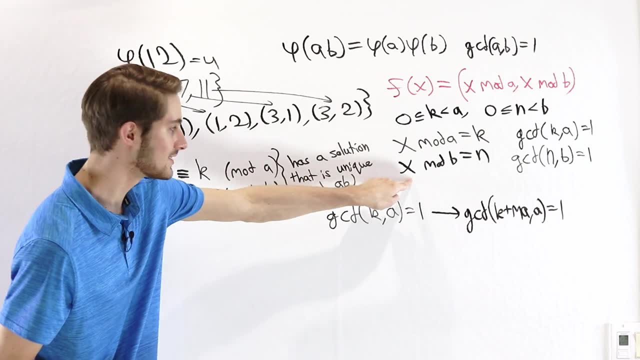 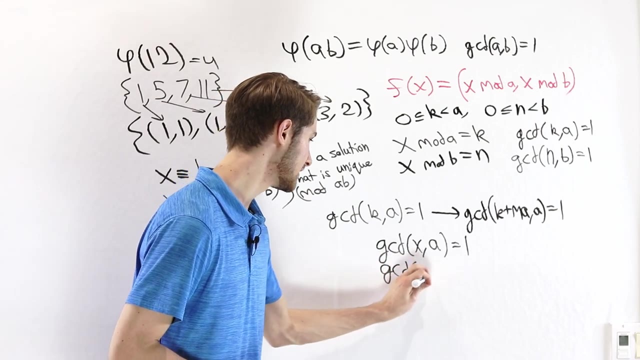 by adding some integer multiple of a. So if k is co-prime to a, then x is also going to be co-prime to a. So we know x is co-prime to a. By the exact same logic we can show that x is also co-prime to b. 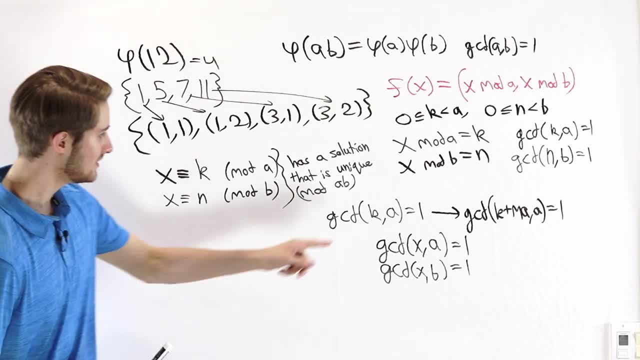 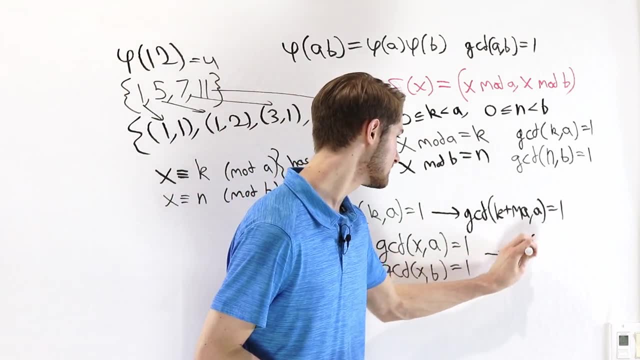 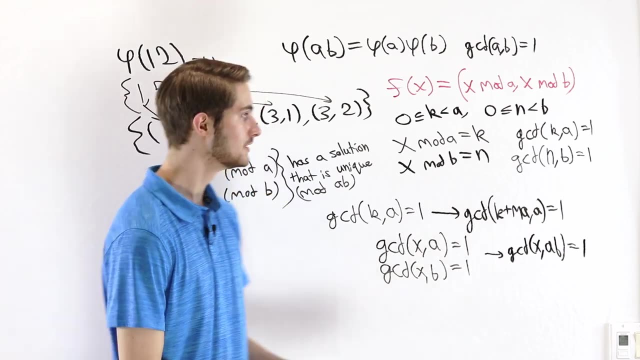 And one of the properties of co-prime numbers is that if x is co-prime to a and x is co-prime to b, then we know that x must be co-prime to a- b. Now this is super important because the first set we're looking at here 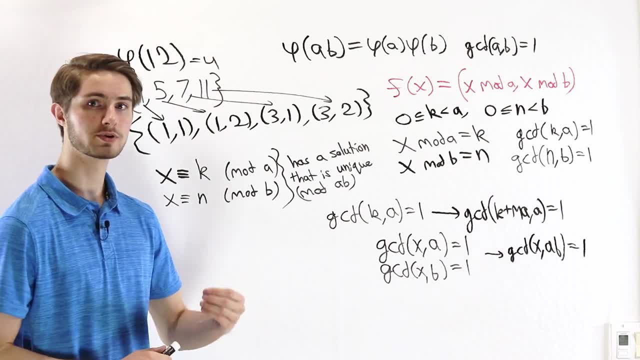 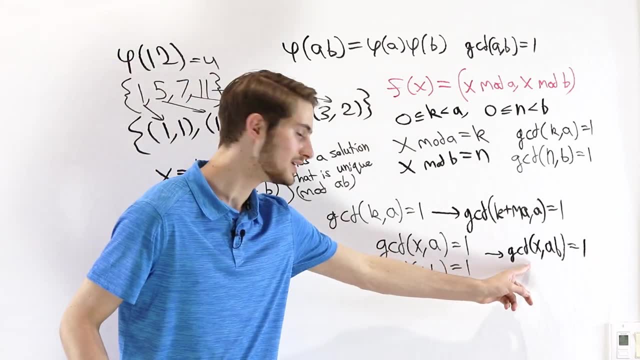 is the set of all numbers that are co-prime to a b between 0 and a- b. So we know that we can find a solution- x- and that that solution is going to be co-prime to a b, But in this first set. 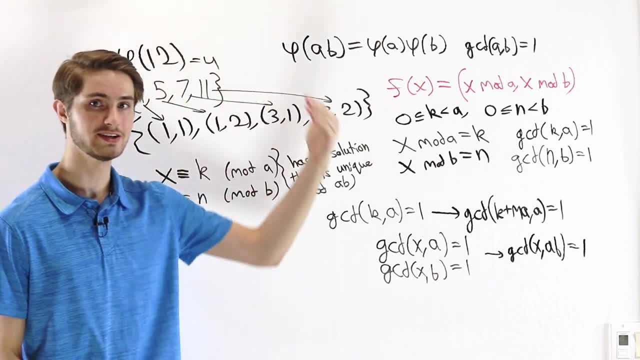 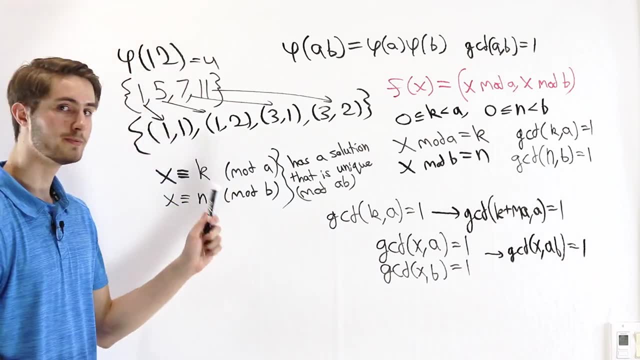 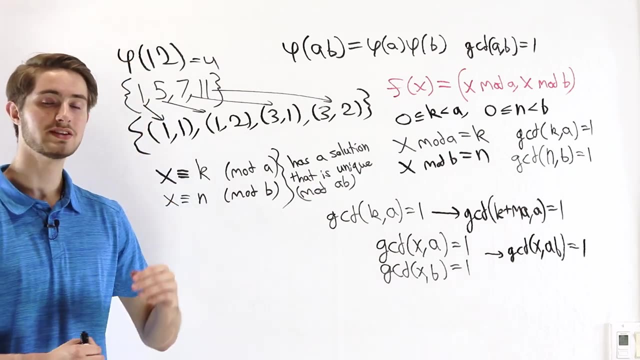 we also know that the numbers are between 0 and a- b. Can we specify that for our number x? We actually can, because we know by the Chinese remainder theorem that the solution is unique mod a- b. What that's saying is that if we add a multiple of a- b, 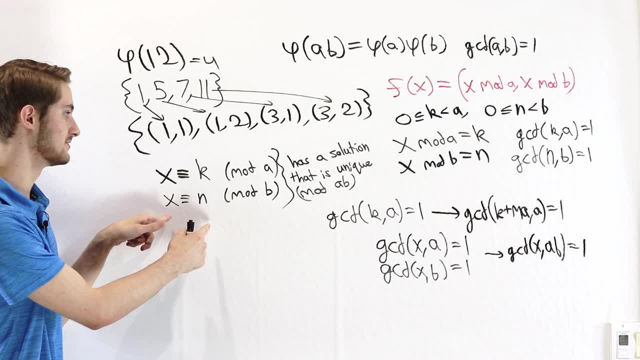 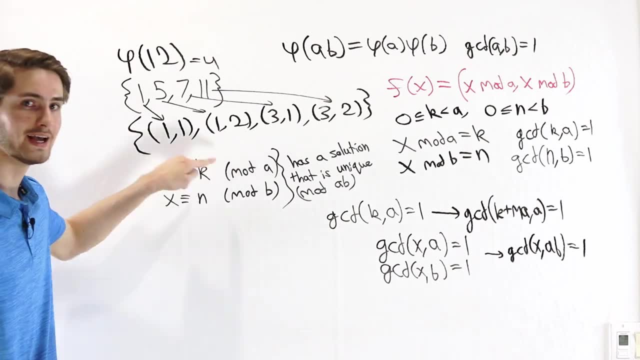 it's still going to be a solution to both of these congruences. And that makes sense because any multiple of a- b is going to be congruent to 0, mod a and mod b. So if we get a solution, x, that's bigger than a- b. 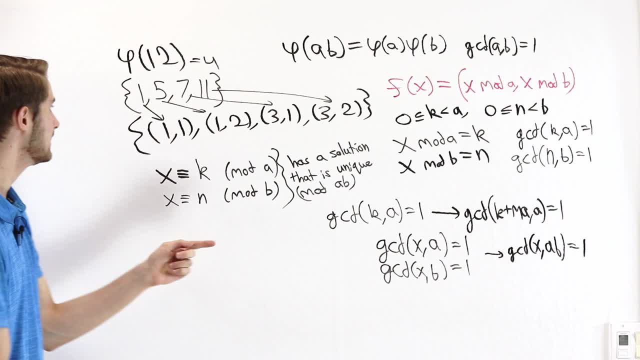 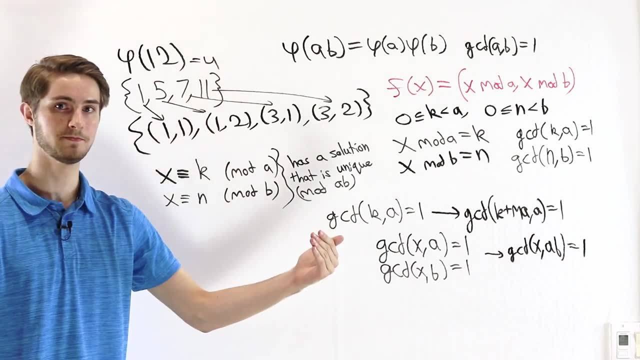 we can reduce it mod a b and get a number in this set A number co-prime to a b. that's between 0 and a b. So how does that relate to our initial question? We're trying to show there's a bijection. 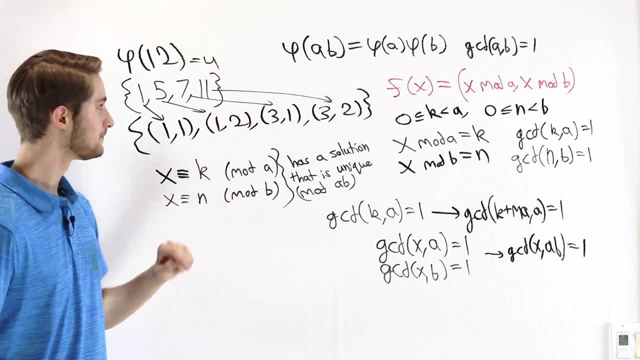 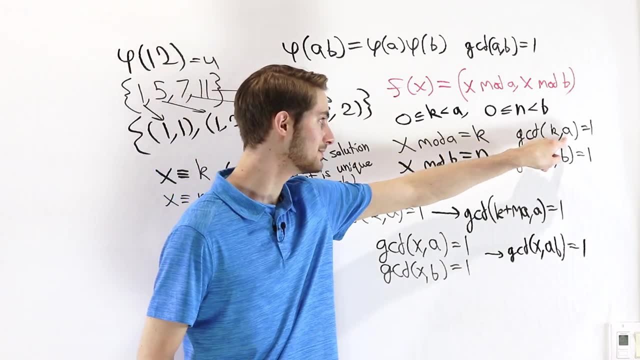 between these two sets. What we just showed is that for any ordered pair in the second set, for any pair of numbers where the first is co-prime to a and the second is co-prime to b, we can find a solution in the first set. 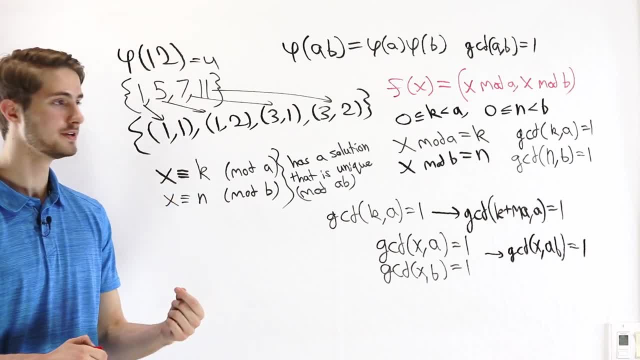 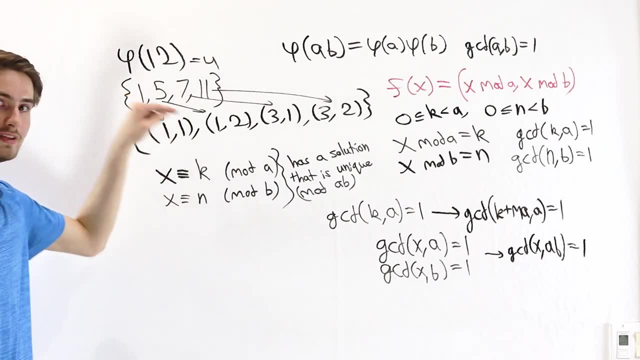 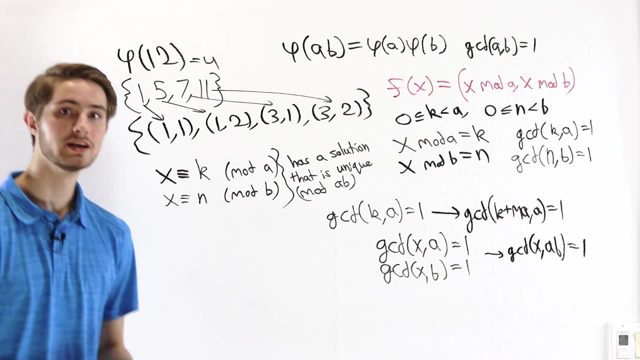 Now, because there's always a solution for every output in the second set there exists at least one input that gives that output the correct ordered pair. We know that the function mapping x mod a, x mod b, that is a surjection. 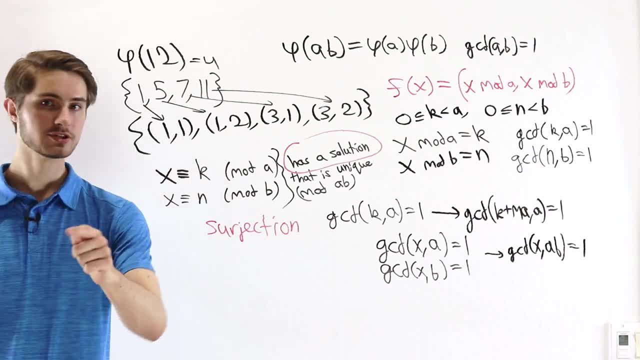 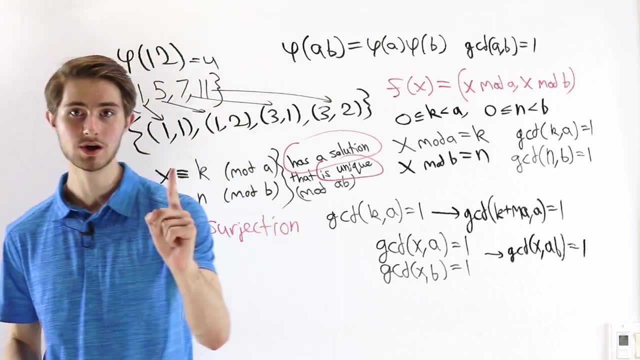 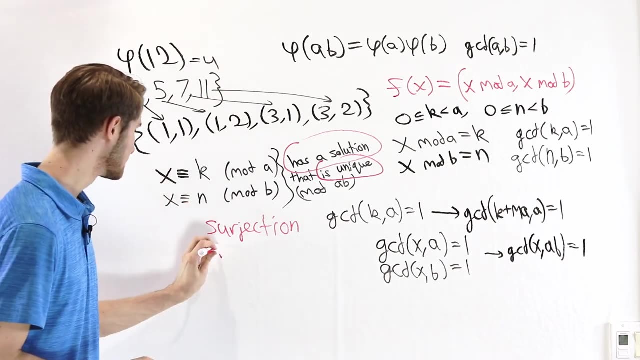 And the Chinese remainder theorem also says the solution is unique mod a- b, which means there's only one number between 0 and a- b. that solves this system of congruences. What that means is that the function is also an injection, And because of that, 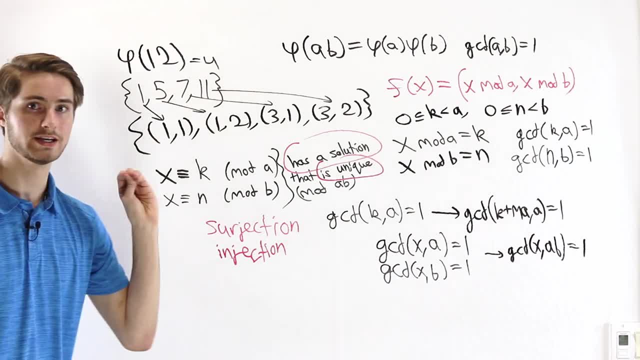 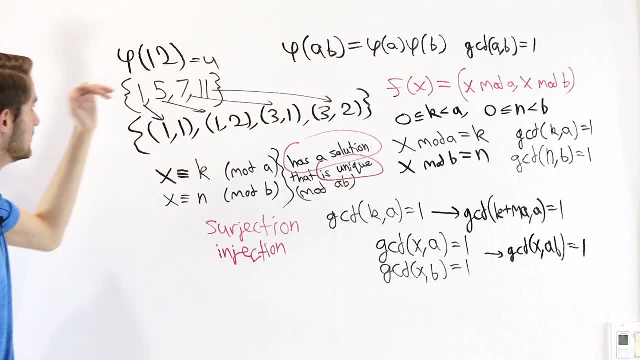 we know that this function has to be a bijection And because the number of elements in the first set is 5 a, b and the number of elements in the second set the number of these ordered pairs, where the first is co-prime to a.